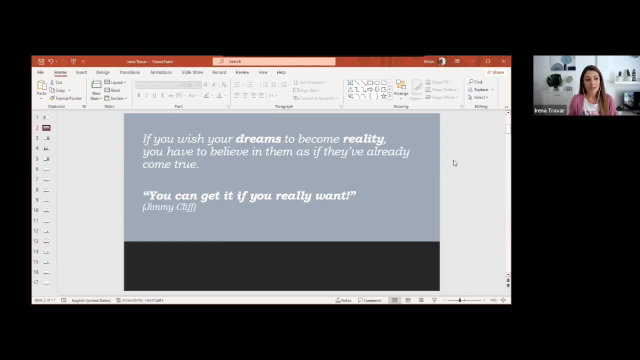 I wanted to share something with them. Actually, this is something that is my motto in life, So if you wish your dreams to become reality, you have to believe in them as if they've already come true. So, actually, I will tell you later something about my experience and my educational background. 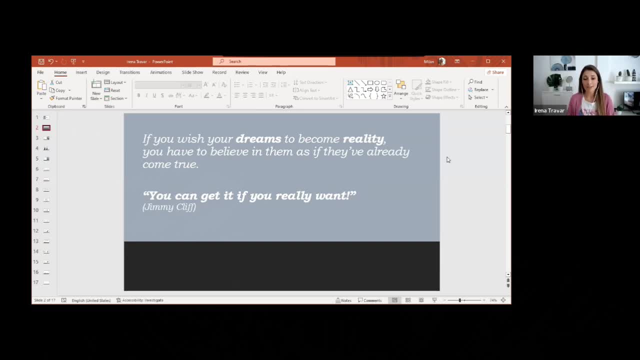 and you will see that, Actually, you can never predict the circumstances, so you need to be adaptable and you need really to believe in your dreams. For example, my wish was always to come and live in Spain. That was impossible for me, for example, 10 years ago, but actually, I think, three years. 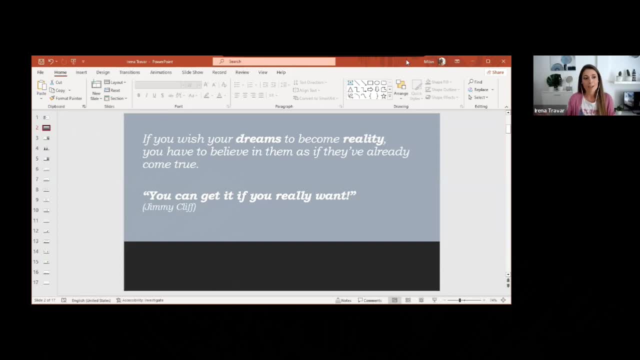 ago- yeah, three and a half years ago- I moved to Spain. So actually everything is possible. And also I want to share something. One of my favorite songs is from Jimmy Cliff, so you can get it if you really want. 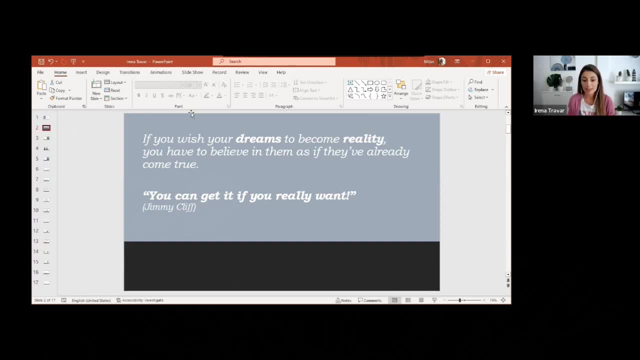 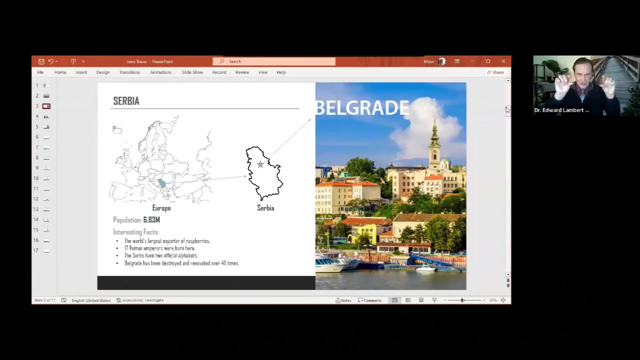 So, of course, just believe in yourself and really you can achieve everything that you want, even though, for example, at that moment it seems impossible to you, but everything is really really possible. Okay, so Can I ask you to minimize the menu up top so that you're there, you go. 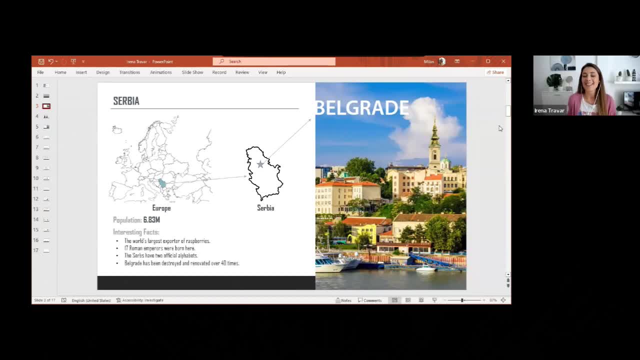 There, Yeah, Perfect Like this. Okay, Thank you, Okay. So first of all, I would like to share something with you about my country of origin. Actually, I always like to present myself so that you know, You know who you are, who you are talking, talking to. 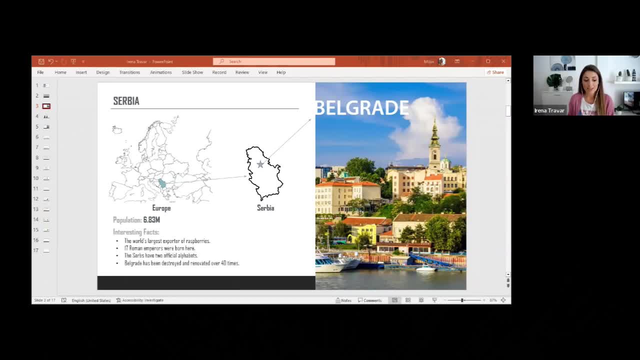 So this is some. these are some interesting facts about the country where I was born and where I was raised. So it is Serbia, in the southeastern part of Europe. So it is very small, landlocked country. It has almost 7 million inhabitants. 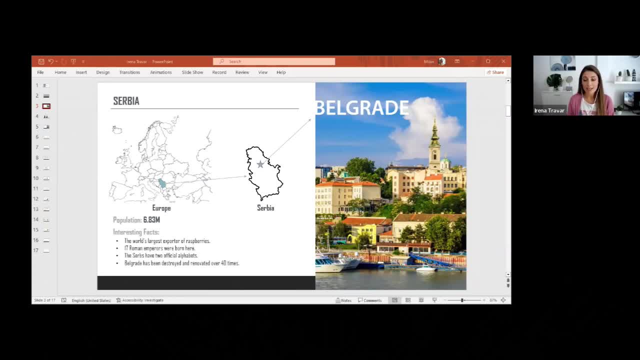 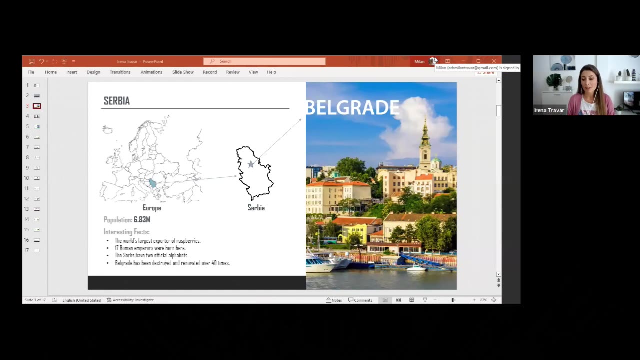 So very, very small population. The capital is Belgrade, that you can see in In this photo, But actually, even though it is very small country, I would like to mention some interesting facts. For example, we are the world's largest exporter of raspberries. 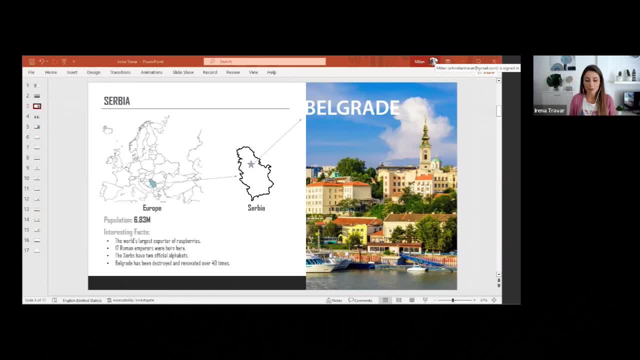 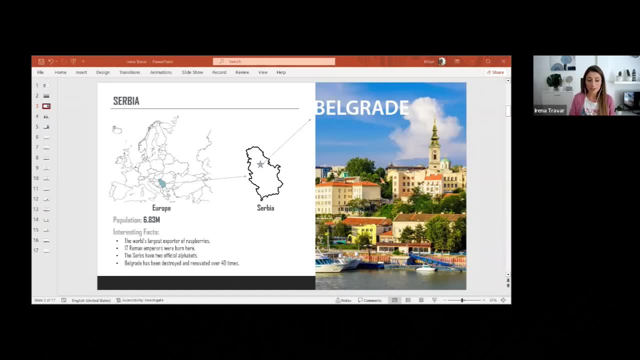 So we like to say, for example, that we have a red gold. For example, around about 10,000 tons of raspberries are handpicked annually from family orchards and exported worldwide. So that's why we say That we have a red gold. 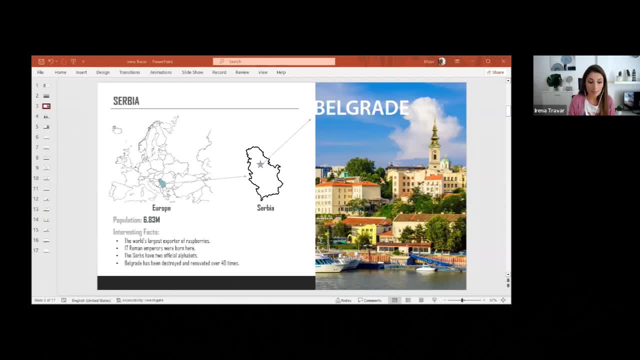 Another interesting fact is that 17 Roman emperors were born here, because the territory of the modern Republic of Serbia was a developed Roman center. So there are numerous archaeological sites across the country that are very interesting for tourists who come and visit them. For example, I was also working as a tour guide. 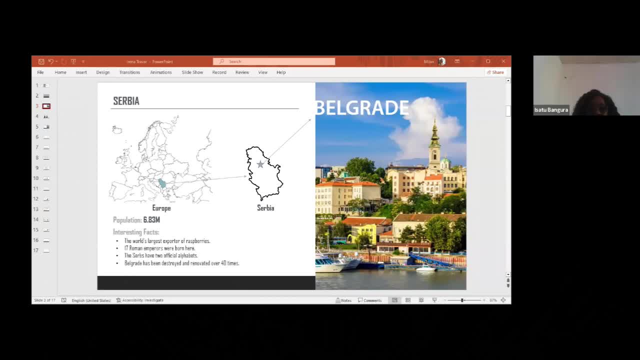 So I can tell you really from the first hand. It's very interesting to all tourist because they don't expect that when they travel to such a small country in Southeastern part of Europe. Also, another interesting thing is that we have two official alphabets. 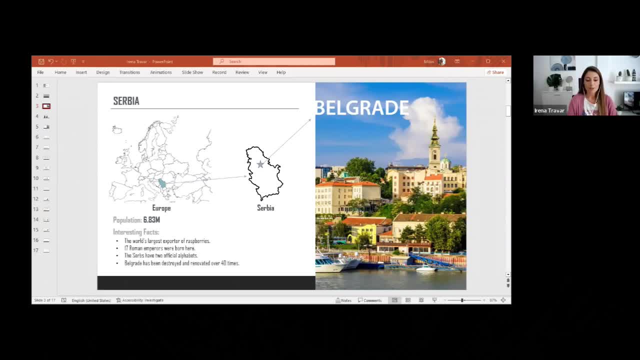 So we have Cyrillic and we have Latin. Cyrillic alphabet is more common for Eastern countries like Russia, for example, And in Serbia we use both. Cyrillic alphabet is more common for Eastern countries like Russia, for example, And in Serbia we use both. 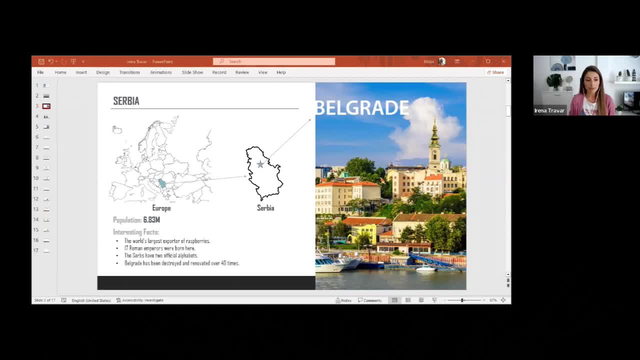 Cyrillic and Latin. Cyrillic is our official letter, but we can write, of course, perfectly Latin. So also what is interesting, that Serbia was part of ex-Yugoslavia. And, for example, if you travel to other countries like Bosnia, Croatia, Bosnia, Montenegro or even North, 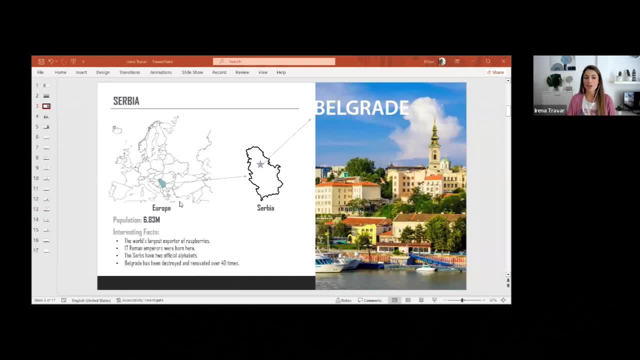 Macedonia. we can perfectly understand each other. We can say that we speak the same language, So our alphabet is very consistent. For example, we had one reformer in 19th century, Vuk Karadzic, who came up with the concept: write as you speak and read as it's written. So we have. 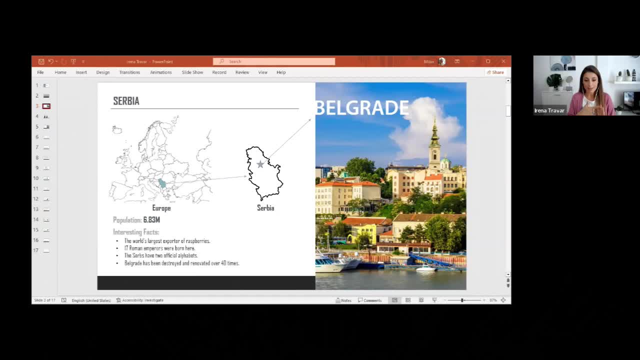 one letter for one sound, So it's like perfect language. There are no other languages in the world that are like Serbian. And also another fact is that Belgrade has been destroyed and renovated over 40 times because of its almost perfect geographical location in Europe. It's located at the confluence of the two rivers Sava. 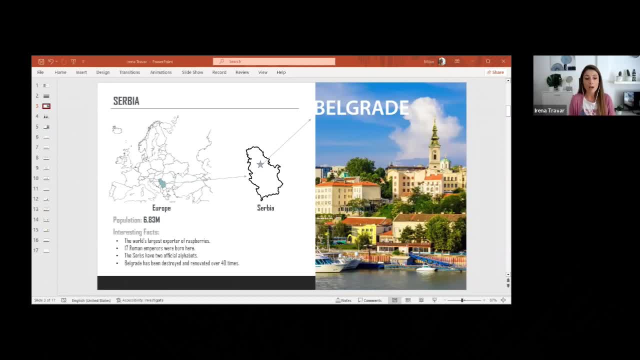 and Danube. Danube is the second longest river in Europe And also the city is located exactly when Pannonian Plain and Southern Mountains meet- So perfect geographical location. And it was destroyed more than 50 times. So that is the reason why we have today very, very 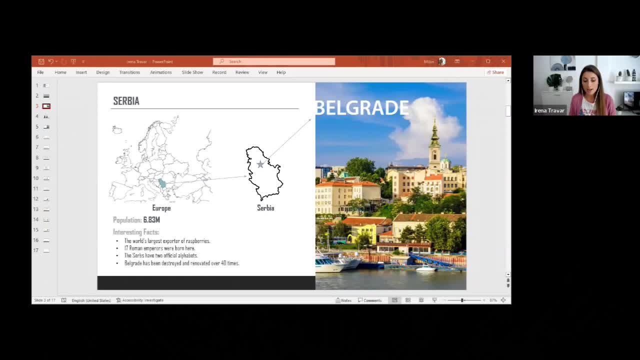 important. We have a very diverse architectural style And also we have different influences in our tradition, in our culture, in our food as well. So, even though it's a very small country, I would like also something to mention to you that's also. 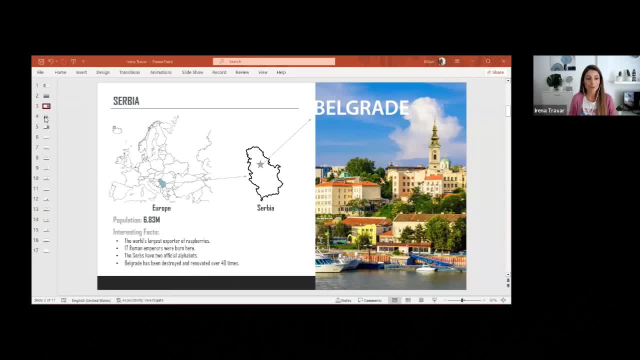 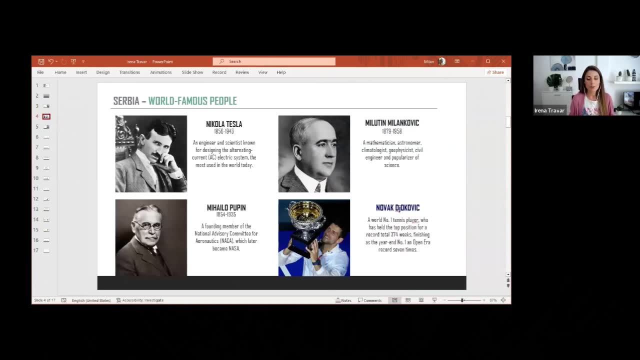 very interesting for tourism if you travel to this part of Europe. So we are really proud of some famous people who are Serbians. So we are really proud of some famous people who are Serbians. So the first one that I would like to mention is Nikola Tesla. So I think everyone heard about. 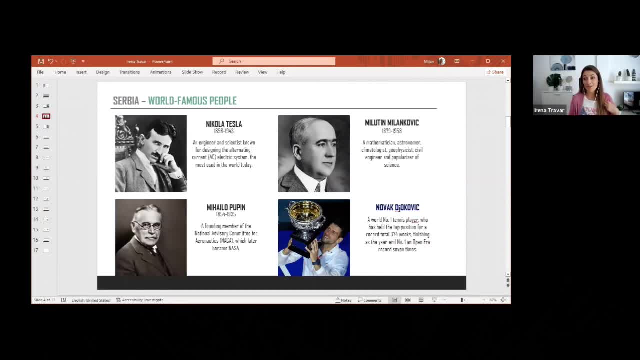 Tesla, But maybe many of you don't know. actually, for Nikola Tesla, You know electric vehicles that are synonym like Tesla, electric vehicles, But it is the surname of one famous scientist, So who was an engineer, a scientist and who invented theleh electric systems that we use today. So actually his inventions were like: 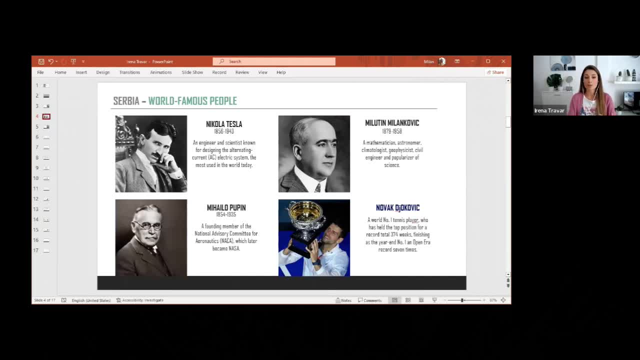 remote control, radio, wireless communication. So that is the reason, so how we can communicate nowadays. So actually we can be different parts of the world. Everywhere in the world we can communicate thanks to Tesla's inventions. So actually, Serbians, we are very, very proud of. 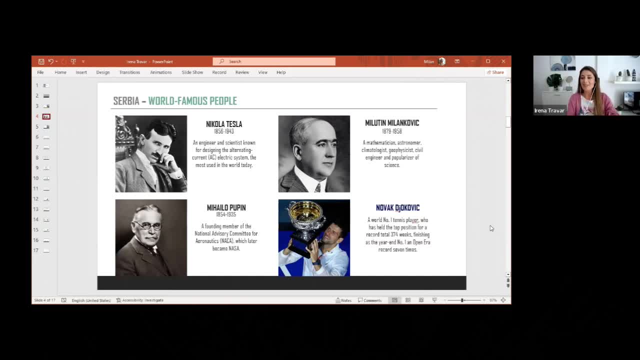 him, and we always like to emphasize that- that he is from our country, uh. the next one that i would like to mention is milutin milankovic. it's a. he's a mathematician, astronomer, climatologist, geophysicist, civil engineer and popularizer of science. uh, so he concluded, for example, that: 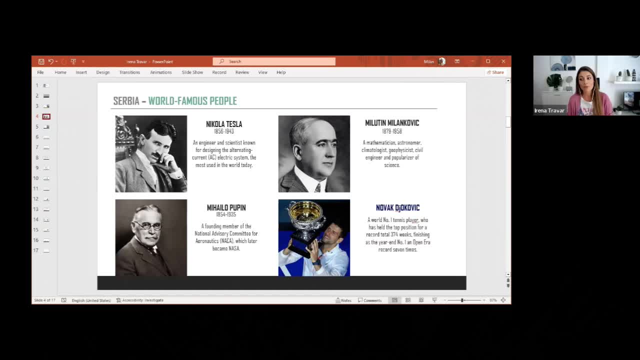 earth's orbit changes in three cycles of different lengths. so that is one of his most important theories. and uh, the third one is mihailo popin, founding member of a national advisory committee for aeronautics, and it later became nasa. and the fourth one, which actually we are very proud of. 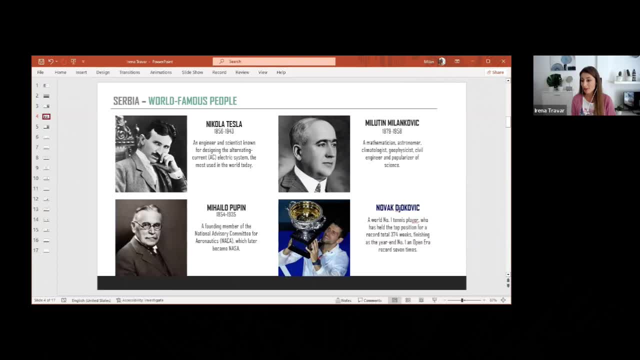 is a famous athlete, novak djokovic, world number one tennis player, and this picture is for, from his last tournament in australia, grand slam, um which, which he won. it is uh. it was his tenth time that uh, that he won australian uh open, uh, so that was something. 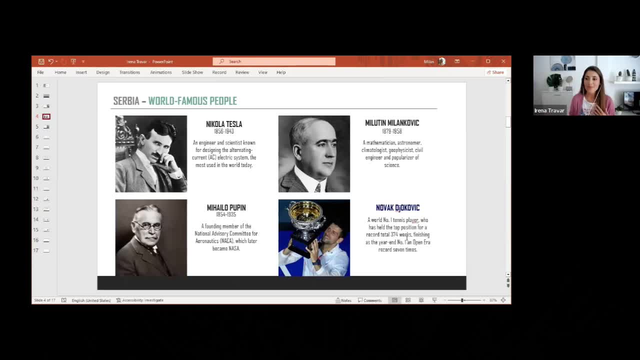 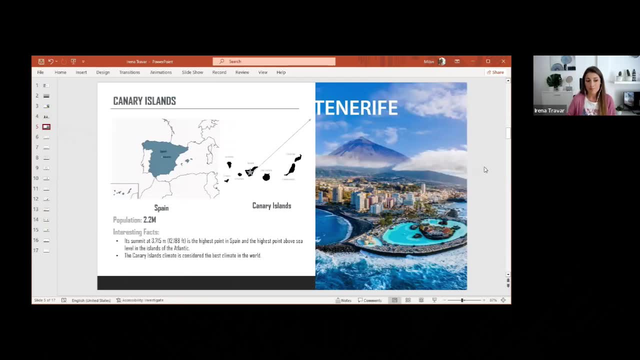 about the country where where i am uh. i'm from uh and now i live in uh canary islands, so they are uh part of spain. the island where where i live is uh tender reef that you can see on the picture. this is um. this is puerto de la cruz, one of the cities in 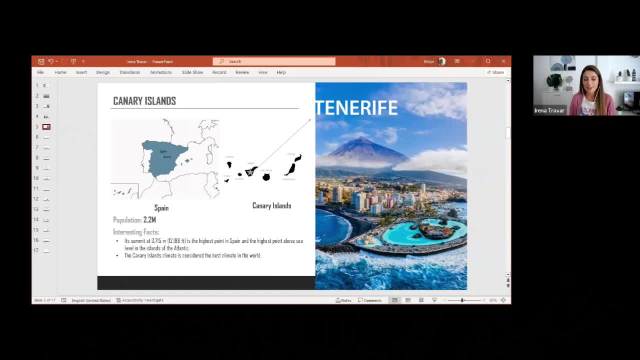 south, in the northwestern part of the island, and you can also see mount teide on the picture. so the islands are volcanic islands and uh, the last eruption of mount teide happened uh more than 100 years ago, in 1909, when uh one city in the 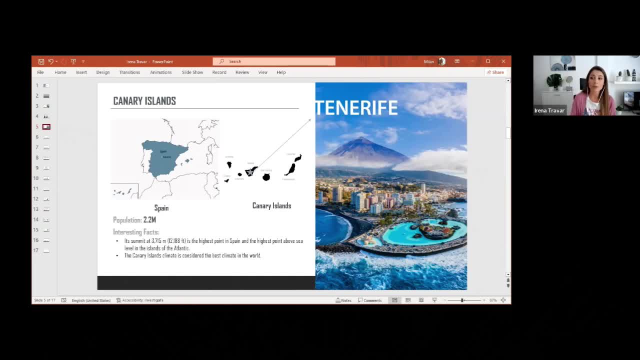 southwestern, in the- uh yeah, in the southwestern part of of the city was completely destroyed. only one church survived, that was. that is very, very interesting. um, so actually the last eruption of all the canary islands happened only a year ago. it is the island that is a hundred. 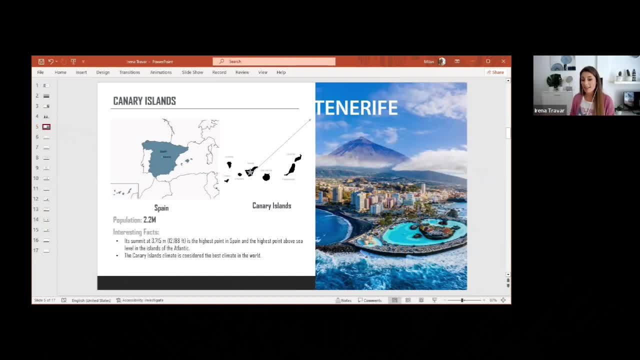 kilometers far away from tenerife, and it is la palma. maybe you you've heard about, uh, that that eruption, uh, so, uh, this is also, uh, mount teide, the highest point of spain and also the highest point above sea level in the islands of the atlantic. uh, also, another interesting fact is that canary. 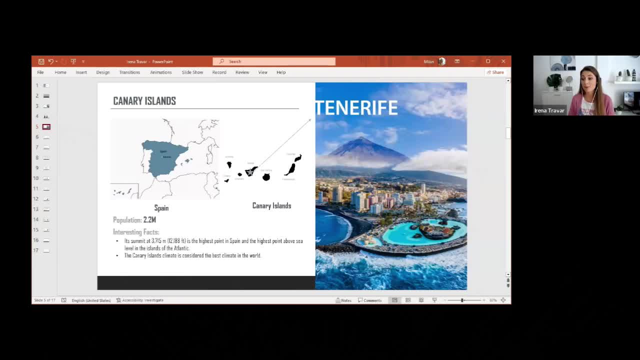 islands climate is considered the best climate in the world. uh, so actually we have really um nice summers with degrees around, with the temperature around 30 degrees. it's very rare that it's above 30 degrees, just sometimes when we have, for example, kalima, that is. 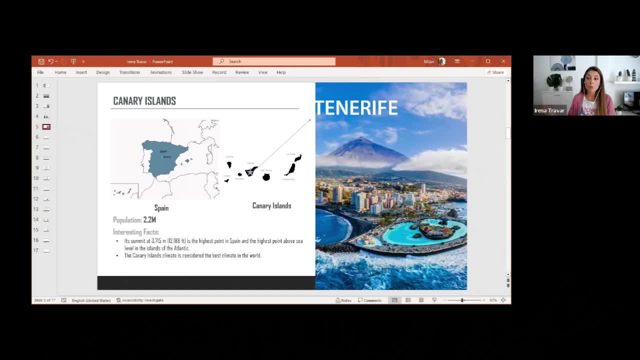 um, weather condition when there are strong winds from africa, uh, and then temperatures can maybe be 35 degrees, something like that, but it's not very common. if it happened, maybe. if it happened maybe one, one week or two weeks during during the summer also- now it's winter, but actually it's. 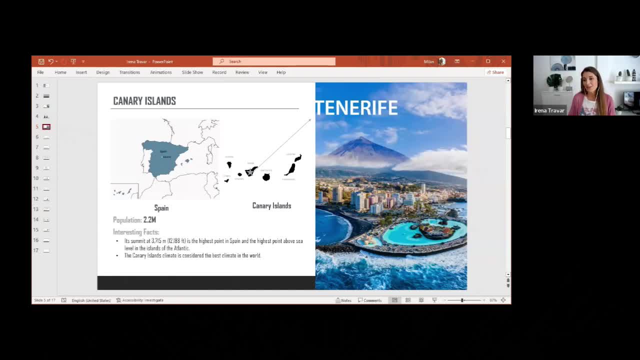 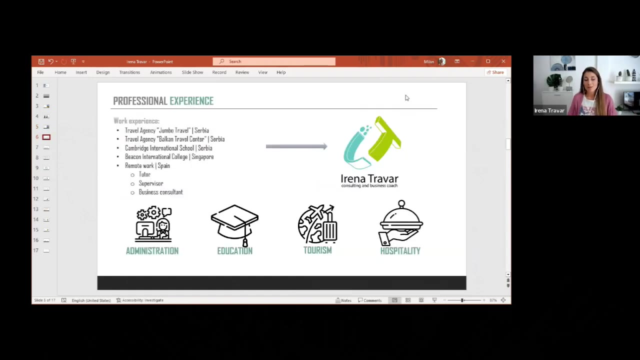 around the- i think, 20 degrees uh outside, so actually it is a perfect climate, and that's also one of the reasons why i decided to come to the canary islands, uh and uh, and live here, uh. so something about my professional experience. well, i started my professional career in serbia. 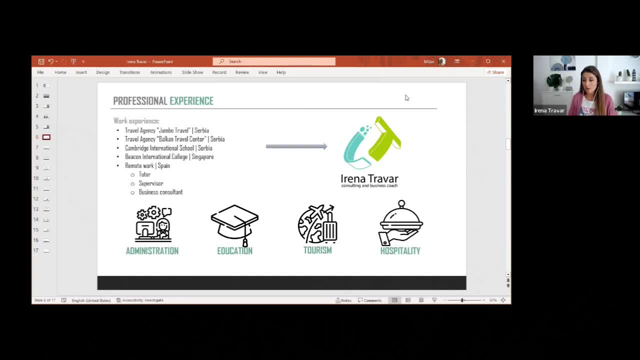 uh, so i, um i- worked for two travel agencies. first, in the first travel agency, that is, jumbo travel, I worked as a tender project manager, so actually that means that i was one of the person who was responsible for participating in all tenders, uh, that were related to, uh, selling. 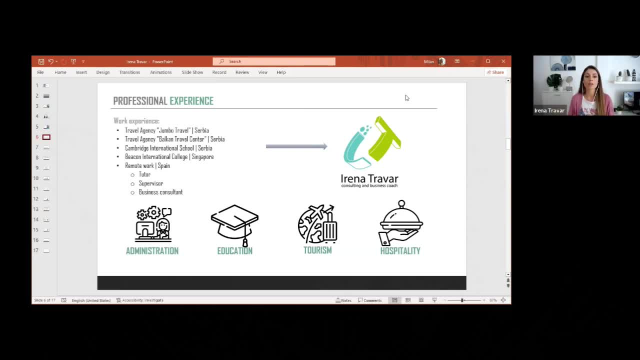 flight tickets and the hotel accommodation for the whole world, because, uh, in, in jumbo travel, we with um, we sold uh flight tickets and also hotel accommodation for the whole world, uh, so actually that was a very challenging for me because that was my, my first, uh, my first job, but actually I'm 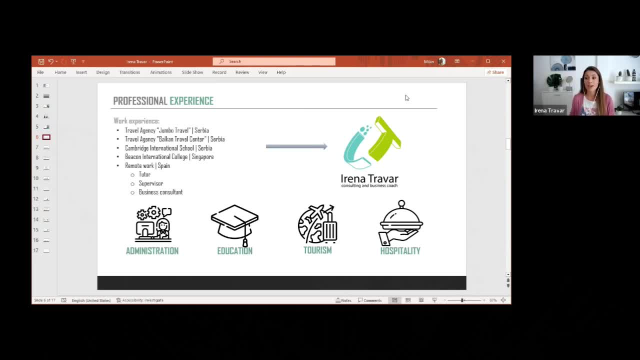 very proud that, um, we won many tenders, that we raised profit. that is, of course, the the most important uh and uh- that we established corporations with many national uh government institutions, for example. after that I also worked as a tour guide in the travel agency Balkan Travel Center. so I have to say that um, 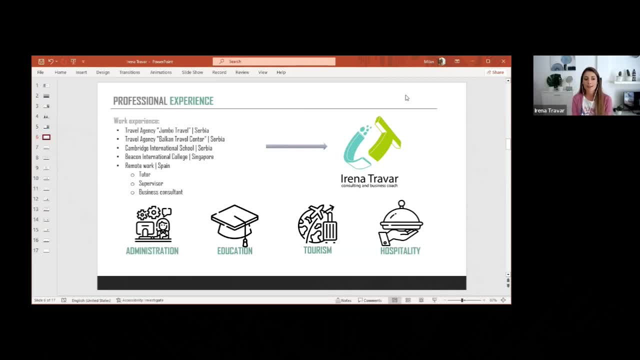 working as a tour guide was, uh, something, uh that I really enjoyed most, because actually you have direct contact with tourists, you are, um, directly talking to, to, to people, uh, so it's not only the part that that you do your research work, for example, and you need to. 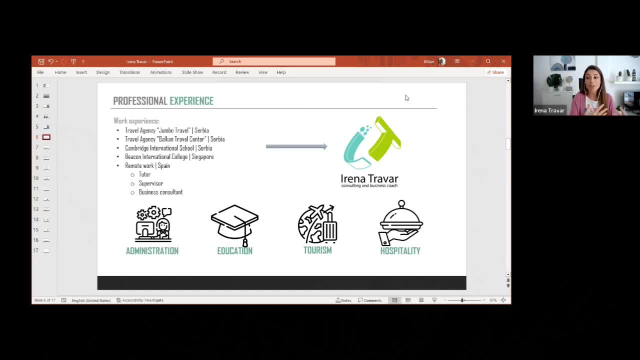 read a lot of literature. you really have to communicate with with people to know what are their needs and wants and to adapt your tours. I also- um, not not only- conducted tours. I organized many tours in- uh, in Belgrade and in in Serbia. so actually tour guiding is really complex because you need to know a lot of things about the culture. 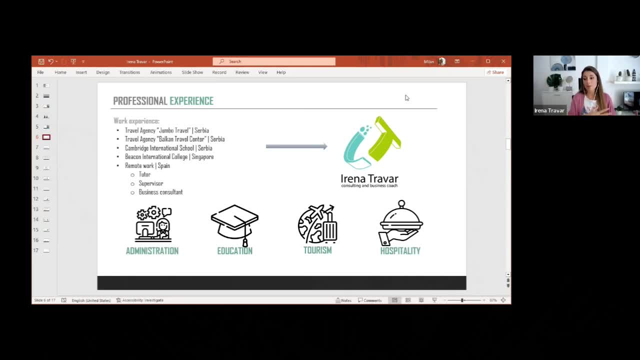 about architecture, about art, about music, so many different things that that can be interesting for tourists, of course, and to know what, what to tell them. so that adaptation to each group, each group was also challenging, but was something that I I really enjoyed, because I like that, uh, communication. 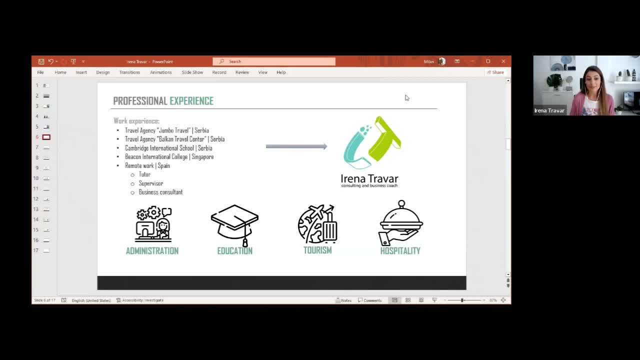 with, uh, with people, and uh, uh, uh, really I can say that, uh, that that were. that was the beginning of my uh entrepreneurship career. uh, so after that, I worked also in one Cambridge International School, where I taught uh Cambridge IDC geography. uh, because uh, I, um I finished uh faculty of geography in Serbia. we. 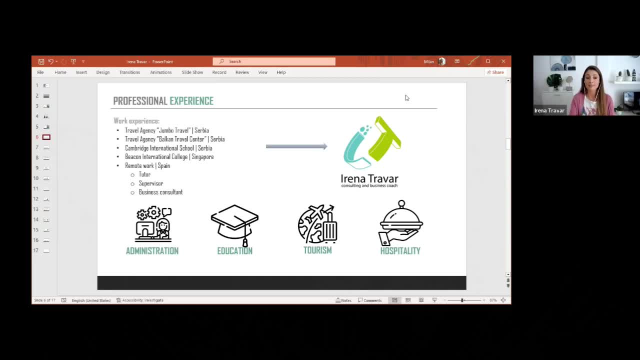 don't have faculty of tourism. we have only one department, that is in the faculty of geography. so actually, when we finish our studies, we can teach geography as well, as well as, uh, tourism, uh, so that was also something, uh, something interesting for me because, as I mentioned, I like that. 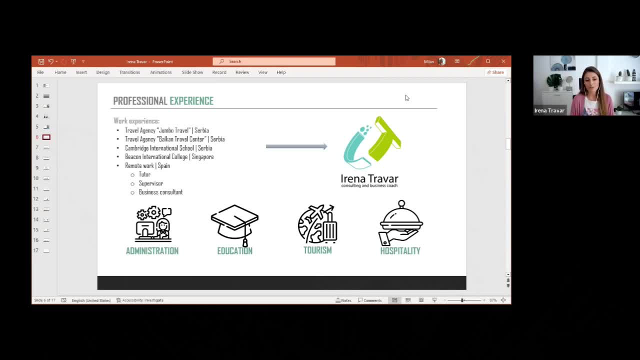 communication with students, with, uh, with people. so for me, it was, uh, it was a really like kind of of a dream job. um, so, uh, after, uh, after that, I moved to Singapore. yes, Dr Ricardo would like to ask a question, I think. uh, yes, of course. oh, we can't hear you, though I don't know why. 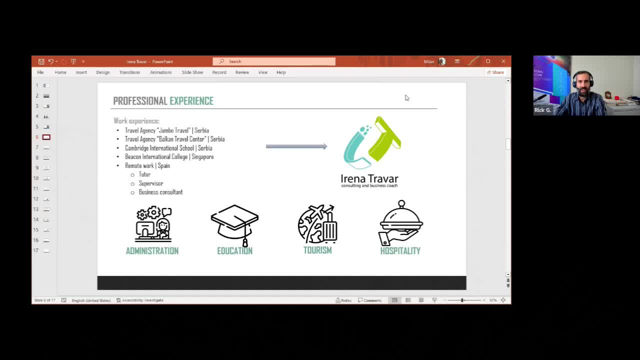 hello, can you hear me now? now I can? okay, fantastic, sorry, uh. yes, Irina, thank you so much for sharing this amazing Journey that that you've been on so far professionally, and I just wanted to share with our students that, um, you know, each of us live in unique places. you know, uh, wherever we are, it's a unique community, a unique 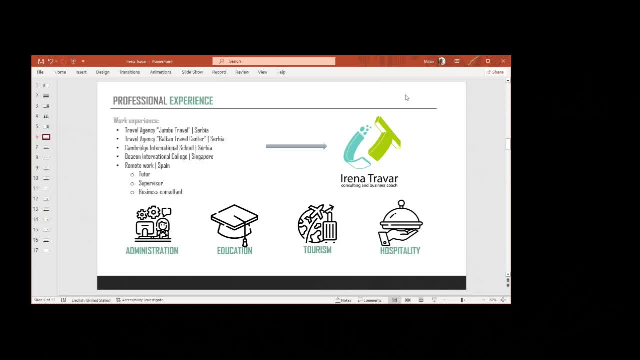 place that we can share the beauty of it with the world- uh, you know, in all of our communities. so I think these ideas that you're giving to us is something that anyone can participate in, and to be a local guide or a local tour guide and to learn from what you, your experiences have been. I 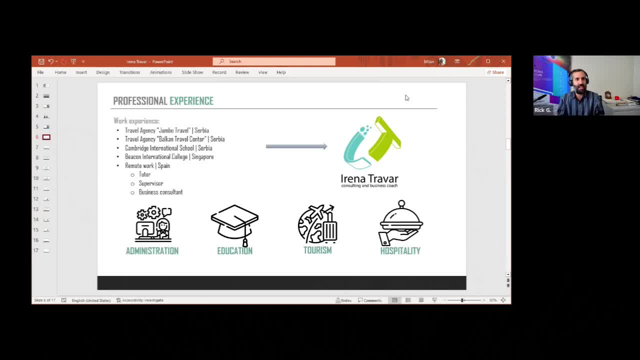 mean there's so many tools today that we have, from Airbnb to uh different uh, you know websites that you can be a tour guide in, and I think you know all of our students are working in different professions, but there's a lot of people who are transitioning from. 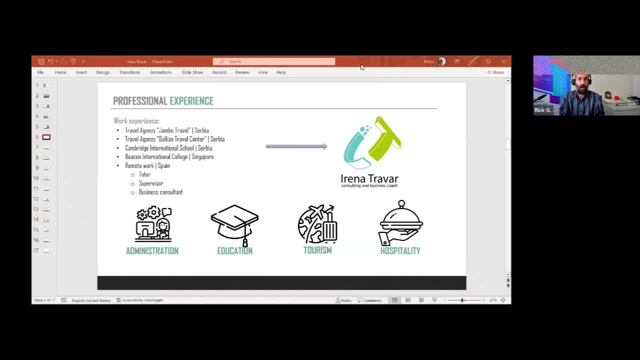 one profession to another, or who would love to have the opportunity to host, uh people in their country, and I can't think of a better person to do that than someone who's been living in the area, who knows the ins and outs, and so it's very interesting that all of us can learn. 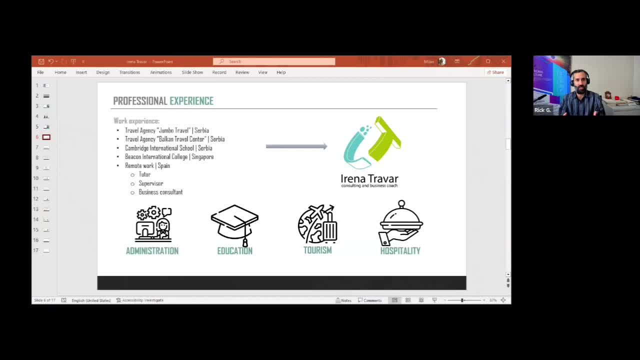 how to participate in this kind of global economy where we can have people come to us and share with us our knowledge of the local cuisine and and opportunities and attractions. so I just wanted to mention that so that all of our participants, which we already have 73, uh watching us, so they 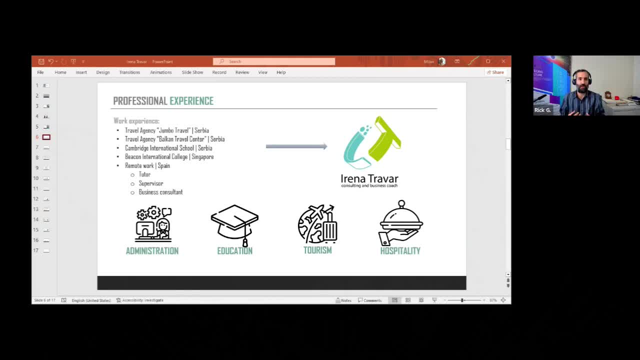 can think of these, these things, as something they can do on their, on their own. um, yes, of course, thank you, thank you very much. uh, well, completely, completely agree with you because you, you can never predict the circumstances and you need to, um, to really uh, adapt your, your. 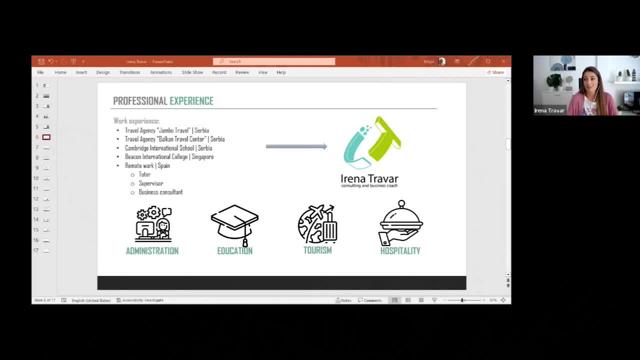 yourself, um, and see what is on on the market and what, what can, can you actually, uh, actually do uh, so, uh, just, of course, it's important to to believe in yourself and don't expect to to be professional at first moment, from the first class, from the first tour or whatever that you do in in your life. 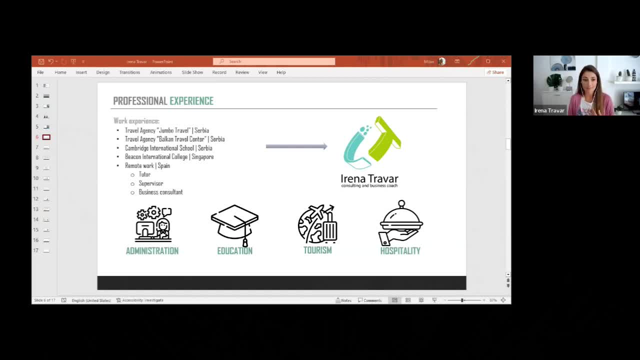 because, for example, when I remember my first tour, uh, really I don't want to remember that. the same thing with my first class, with students, I also don't want to remember, but actually, uh, then you, you really can, can, encourage yourself, because you just need to be aware of your capability, capabilities. 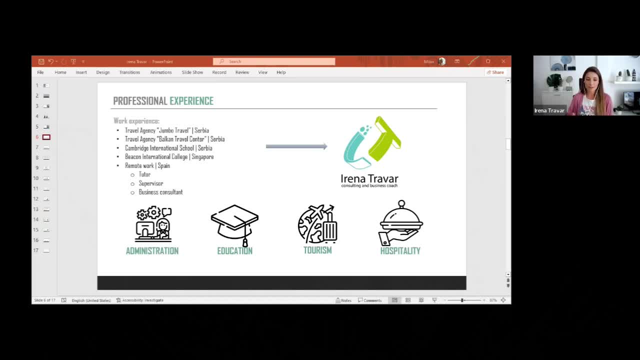 and you, you need to know that everything can be learned and that you need more experience. uh, and you, you can, you then you, then, when you compare your first day and after one year, you can see that there is a huge progress, uh, for example. now I wanted to mention my experience. 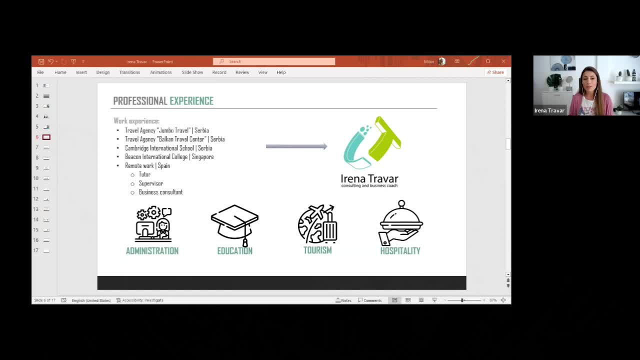 in Singapore when I went, went there, uh, one of my first classes, I think, or or even the first class. I had 70 students in one group, so in one, in one big classroom. so for me that was something I I was thinking, oh, I can't do that, I'll go back. 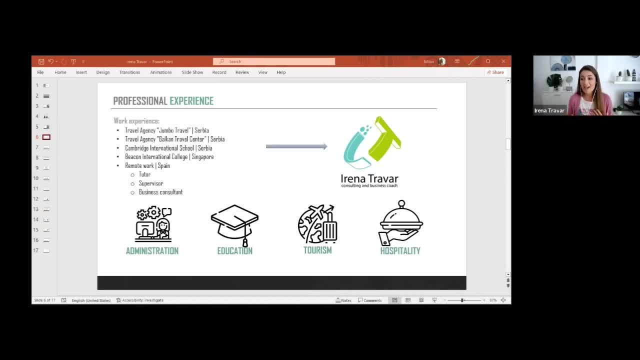 to my country. I'll go back to Serbia. why am I doing that to myself? uh, but actually, when I entered the the classroom, I prepared, of course, all the concept for the lesson activities, so everything, and I always prepare something extra, for example, if I finish something earlier. okay, let's have. 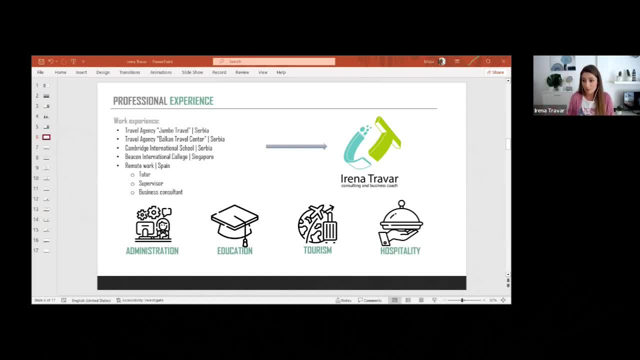 something extra for um, for the end of the class, for example, if we have time, so that preparation is the most important and at the end of the class, really, students were, were satisfied. uh, that was my first class that that really wasn't so bad, like, for example, my first class in Serbia- my very first. 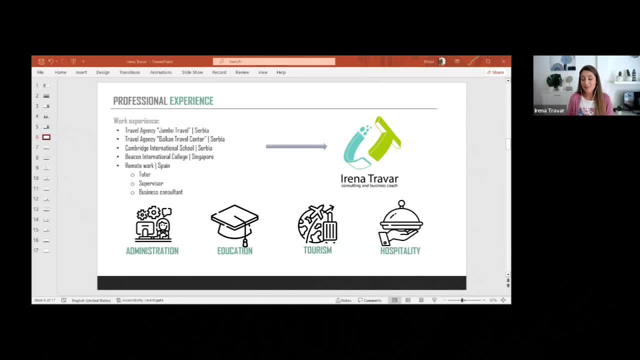 class in, uh, in, in Serbia, uh, so that means that you, you really can do, can do everything, um, and also what I wanted to mention, that, uh, I didn't just receive the offer from Serbia, from Singapore, uh, it's, it's really I, I don't know, maybe if there is one percentage of people who can just receive. 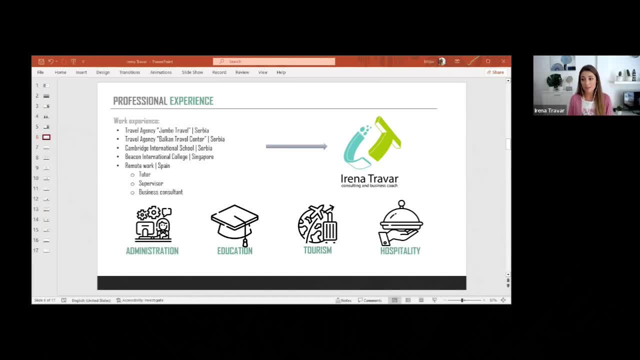 receive the offer. I sent 400 emails to countries like Thailand, uh like um, also Singapore, um Malaysia, China as well, and um I. I, for example, didn't receive any response for a couple of months and I was almost prepared to to give up and tell myself: okay, never mind, I will stay in Serbia, continue doing my tours. 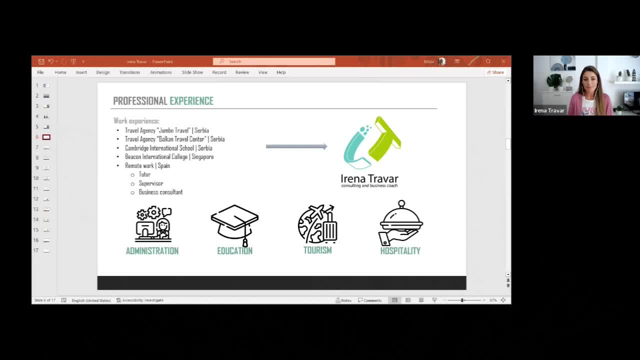 or whatever I was doing, uh, but actually, um, I I felt that I needed more experience, uh, and that's why I decided to, to apply and to to move to Asia. and then I went on holiday and I say, okay, never mind 400 emails. imagine how much time you need to find 400 colleges, schools, 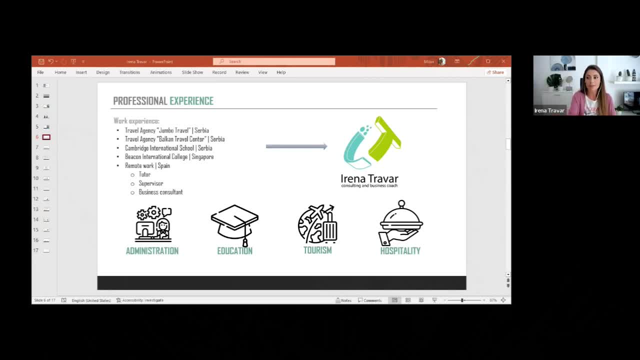 institutions, uh, to find the program where you can teach and to tell people, oh, I'm really ready to come. people don't believe you when you say I'm ready to come, I will come, I will teach them. um, when, when you have online communication with them, um, they don't believe you. actually, how would you come? why would you come? so a lot of questions that. 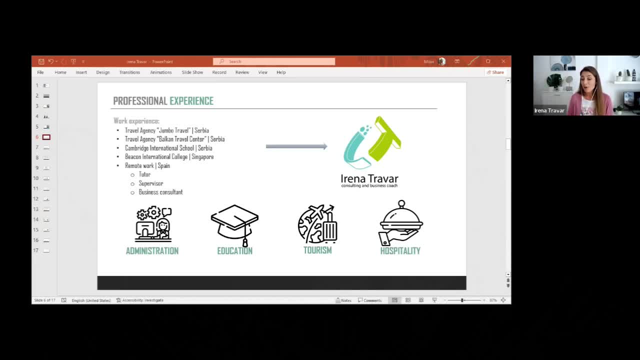 um, that you don't know how to convince them. so I went on holiday and one morning I just received an email from Beacon International College, from Singapore, asking me for an interview, and I was like, oh my God, is it really true? but actually we we already had some interviews before and 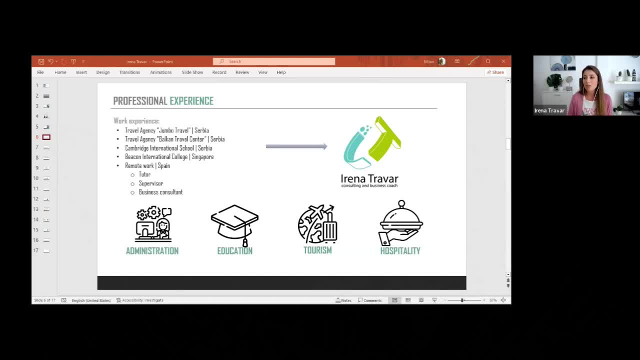 um, I had a feeling that they were not interesting in cooperating with me, so actually I just left it. I received that, that email. I said, okay, but I'm on holiday, I can have an interview when I, when I come back to Serbia. I I really wanted to enjoy my, my well-deserved holiday. then I had a couple 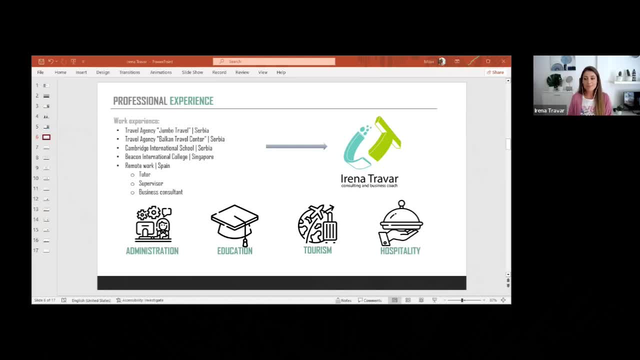 of interviews with them and after three months I moved to Singapore. so actually you can never know what what will happen. you just need to be persistent. so, uh, if you need to send 1 000 emails, okay, don't be lazy. just tell yourself: okay, I will start 30 emails every day and that's it. 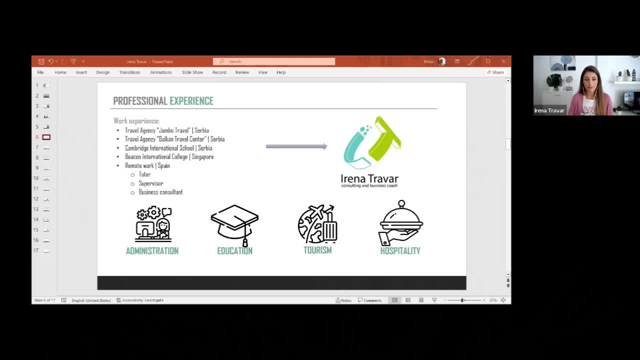 that's what I, what I told to myself: I will not go to bed until I send, for example, 30 or 20 emails. well, it depends, just give one daily goal for for you and follow it. uh, so uh, that was really one amazing experience in in Singapore. uh, but that was Asia and I'm more like. I really like Europe. 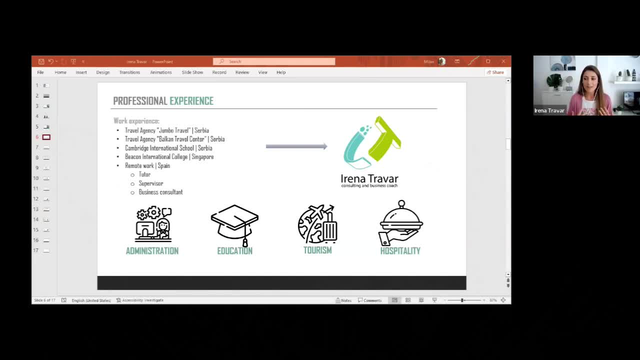 and that Western lifestyle. uh, so I was. I was missing it a lot. I was missing food and, uh, no, everything that is related to to our, um, our Western, Western culture. uh, and even though it was a really perfect experience, I decided to move to Europe, and that 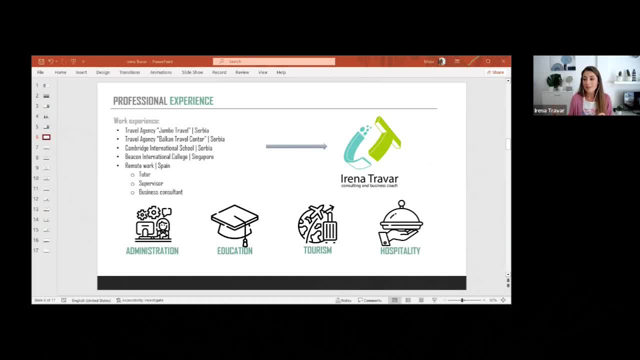 was when I came to Spain and when I really discovered Tenerife, because even though I studied tourism, I studied about Canary Islands also, but when I came here I really could feel that that energy. I really fell in love with, uh, with the island. and imagine: I had no job, I had no house here. 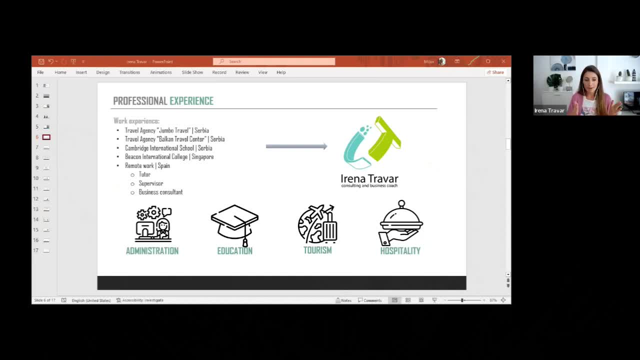 uh, and I said I will stay here. I don't know how, but I want to stay here, uh, so then I said, okay, first I will find some, some apartment and then I will see how, what I can do to to earn money- that is the most important thing- how to stay here. so then I started working remotely, uh, because, 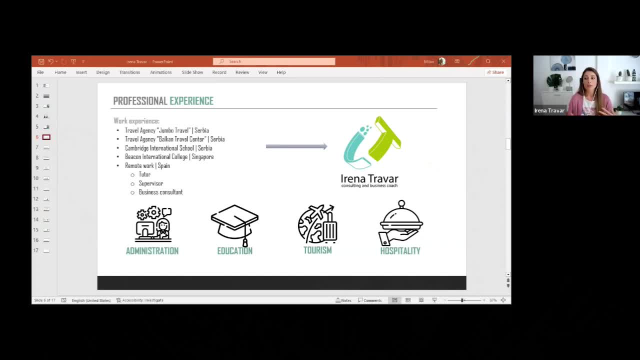 actually, maybe you don't know, but Serbia is not part of the European Union. and then, even though, for example, I had a PhD and I could, I could work anywhere. I could work in one cafe, in one restaurant, never mind, I just wanted to stay, to stay there, but I couldn't find the job because 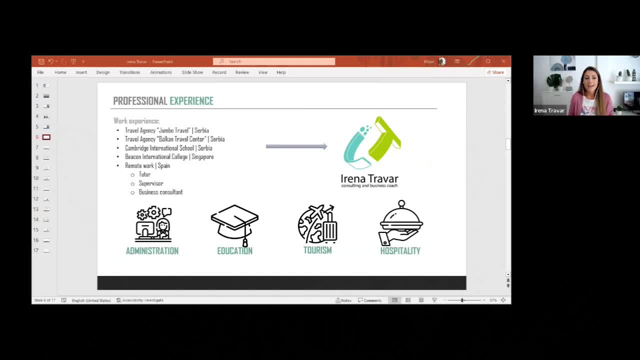 I didn't have Visa, valid Visa- and then I uh, I applied for another type of Visa, but I had to work remotely. I couldn't work in uh here in uh in India. thank you very much, of course, Burke. in Spain, I started working remotely and I created an account on Upwork platform. 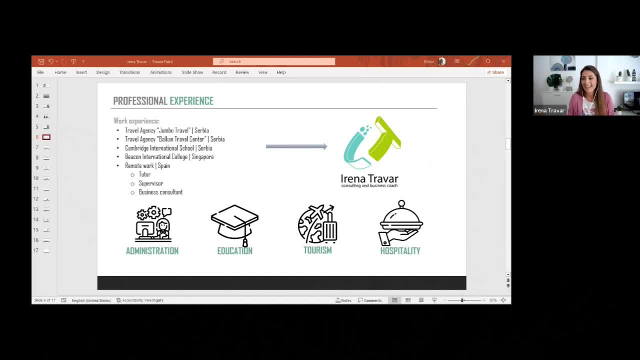 And okay, let's see what will happen. I don't know. Let's start applying for jobs. The first job that I applied, I got a job offer, for example. So you can never know what will happen. For example, my husband was applying one month. He didn't receive any job offer After one month. 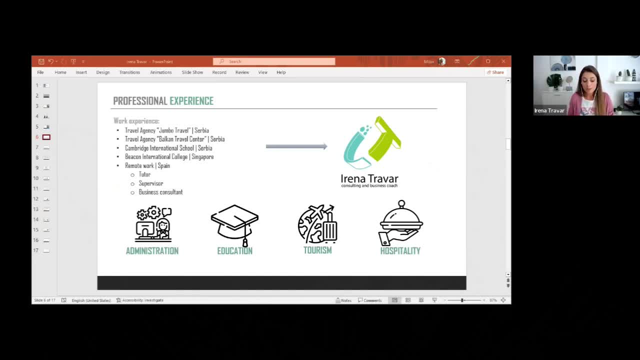 he received, but I received the first one. So that was how I started And I said to myself, oh, it really works, This platform really works. I will continue working remotely. So then I said, okay, what I know to do, what can I do remotely? Okay, well, I'm a PhD, I can do. 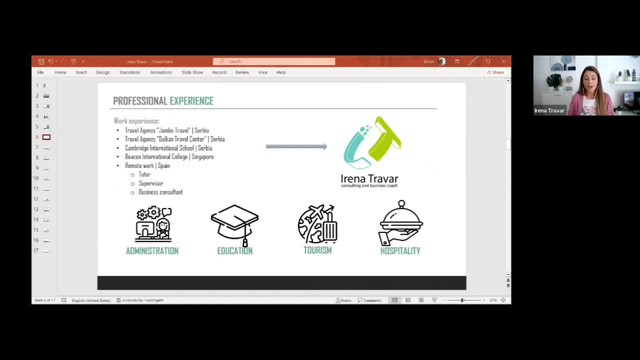 tutoring. I can do supervising students, for example. I can also do business consultations because I know how to do business plans, market research and things like that. So I offered that on On the platform And of course I couldn't earn I don't know how much money, but enough to stay. 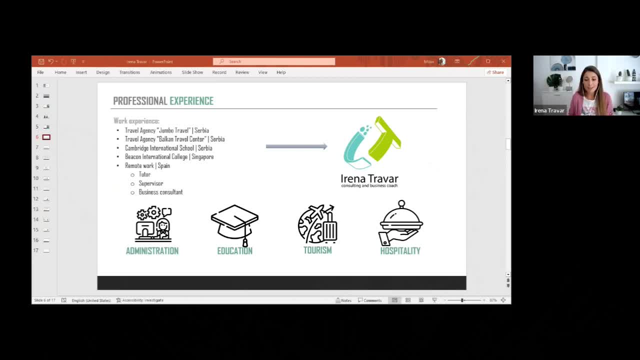 here and to live here. So that is that you really need to believe in your dreams and really work for your dreams. You cannot expect everything to happen. You need to try a lot of things. You know that I mentioned the song. you can get it if you're really, really really. 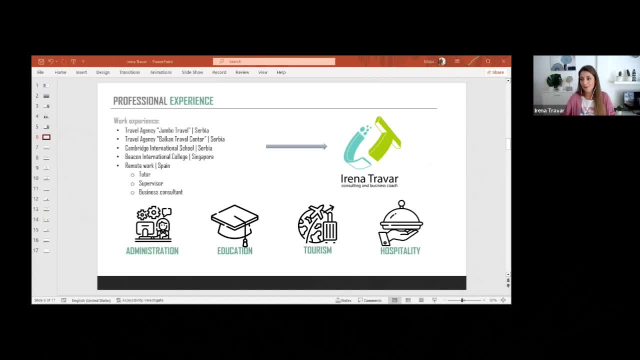 want. Well, it goes on, but you must try, try and try. So, nevermind how much time you need to experience some falls, But of course at the end you will win. So that is something about my professional experience. Yeah, And here I put my logo: Consulting, a Business Coach, That is my. 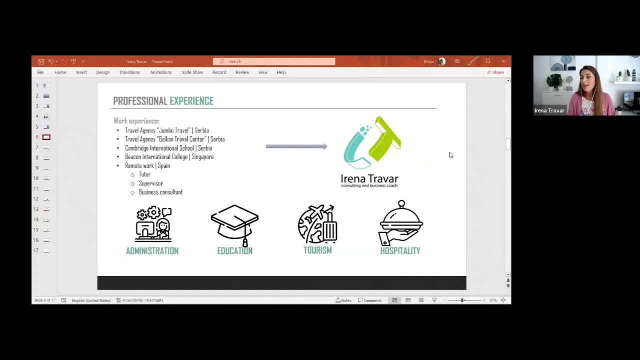 goal for the next couple of months. maybe It's still in the process, but actually I put it here Now. I have my vision, I have my idea, my idea maybe what, what I want to, to, to to come true. I want 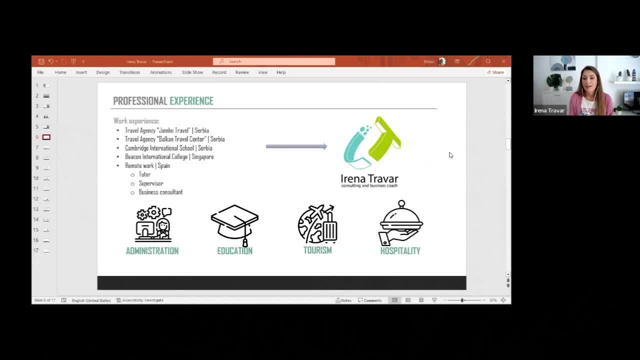 to. to start here, working as an entrepreneur, to have to be consulting and, and and the business coach, because I had many clients on on Upwork. So I gained really valuable experience during these three years. Imagine COVID period, when nobody had work I could work on on the platform. 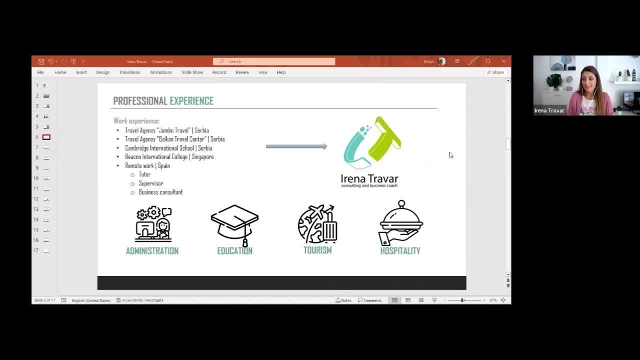 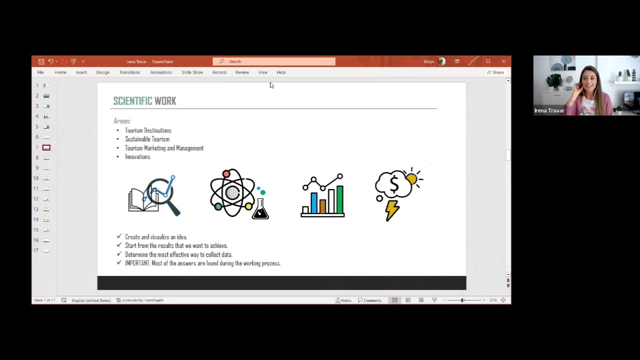 and and survive. Many people lost their jobs, And I also could work remotely, So you always need to find a a way to adapt to to the circumstances. And also another thing that I'm very passionate is scientific work. Well, that is my. 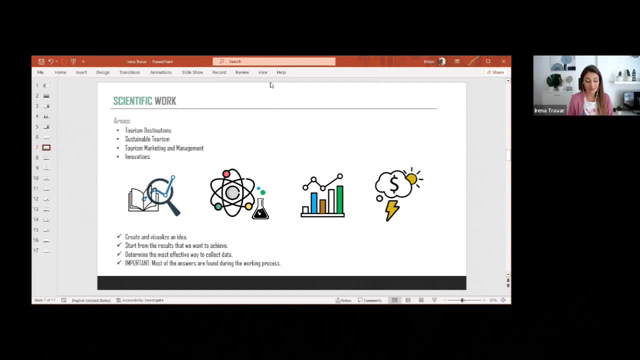 also my, my, my dream, maybe one for the next couple of years, who knows? maybe one year. So I want really to to dedicate to scientific work, because later I will present some of my projects that I'm working on. So, besides my, my professional career, my, my business, 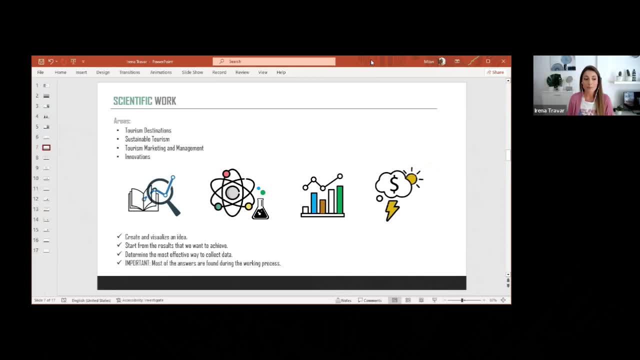 I also do scientific work, So these are the areas of tourism destinations: sustainable tourism, tourism, marketing and management, innovations- So actually everything that is related to technology, to innovations or sustainability is something that that I'm really, that I'm. 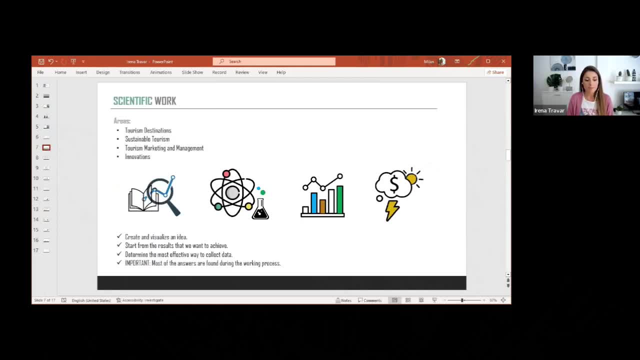 really interested. Okay, I'm sorry, So here I just wanted to to mention because actually you are students and maybe some of you will will start your research career in in the future. So the first what I mentioned here is that you need to create and visualize your idea. So it is important. I need to emphasize that it. 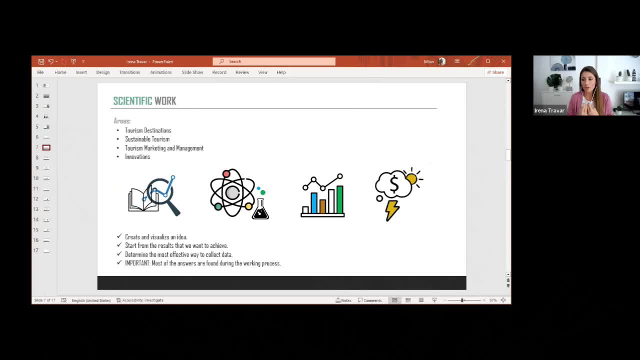 doesn't have to be precisely defined. You don't need to have your conceptual framework at the beginning, where you have only ideas. So this is, for example, something that students always have a lot of doubts. They easily give up on their ideas, but all ideas are really phenomenal. 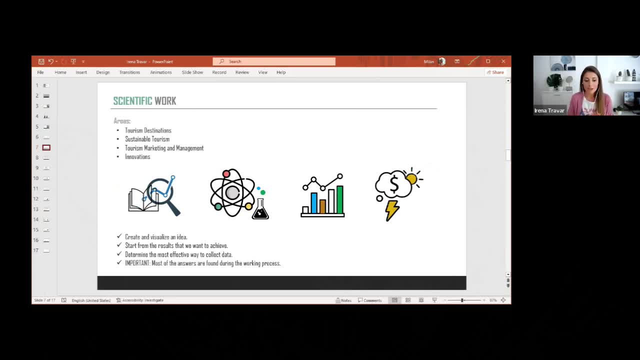 So just just believe. believe in them. So students can. students always have the best ideas, And I remember when I was at my faculty when one teacher told us: now is your time. you need to participate in different projects, You need to do investigation, You need to to have. 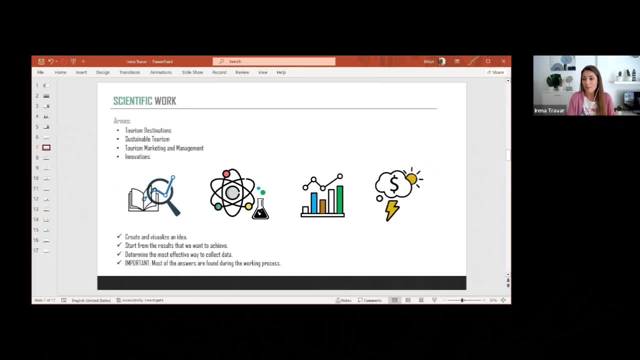 your ideas and and to develop them. And that was like what what she's talking about. I really couldn't, couldn't believe to to my professor because actually I wanted to finish with all exams. I had my scholarship, That was my goal. But now I really understand what that that professor? 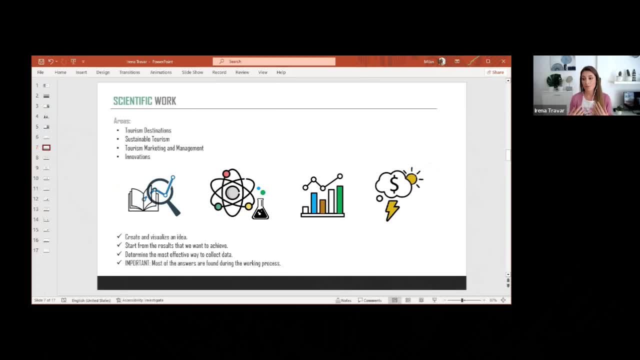 told us. So when you are a student, you you really need to have your ideas and you need to really believe me, you can do. you can do everything. You can have many excellent, many excellent ideas and and, of course, results. So that is, you need to start from the results. 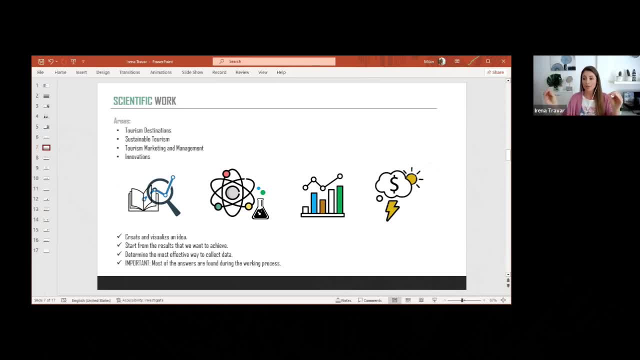 that you want to achieve. So you have your idea and you have the end result. So, even though you don't have a clear idea, you don't have exactly a clear result that you want to achieve, but you have something You maybe want to. you know you want to achieve something, So you need to have your 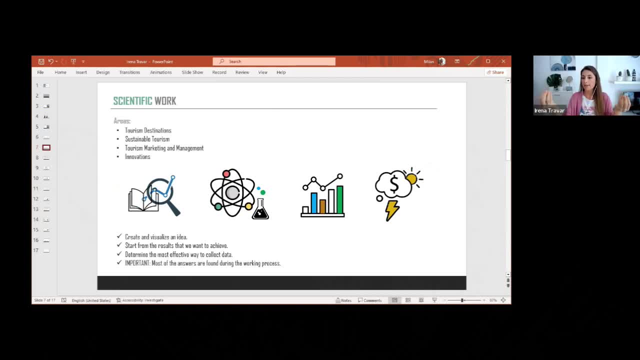 idea and you need to work about sustainability and you want to. your end result is that you want to help. Like my idea was to help small and medium enterprises here in in Tenerife Island. I didn't know how I had an idea, So that is when you need to determine the most effective. 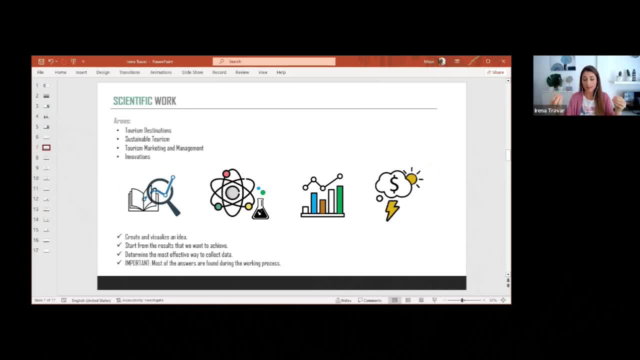 way to connect your ideas with your end result. that is the methodology. So you need to collect data, to do a lot of secondary research and to find what would be what would be the best, the best way to achieve the desired result. Of course, during the process, 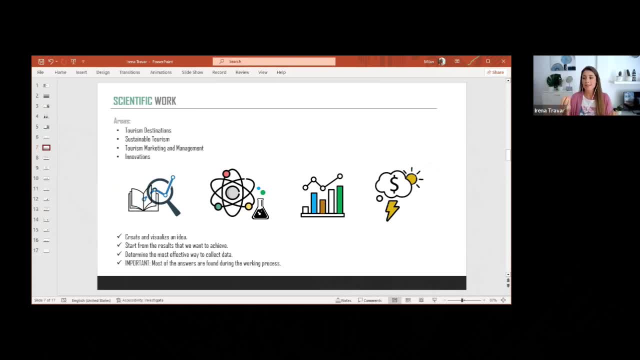 you will learn a lot of things, Some of the answers you will find during the process. So that is why I want to emphasize: don't expect everything to be told to you at the beginning. So just investigate, So give yourself space, give yourself time and really you will. 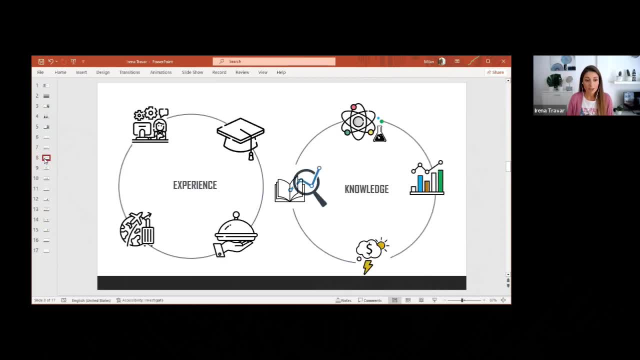 you will be successful. So that is where you need to. you have experience on one side. My experience, for example, are related to education, to tourism, to, to geography, also to administration work, And I also have my, my knowledge. that is from from my, from my studies and also all the research. 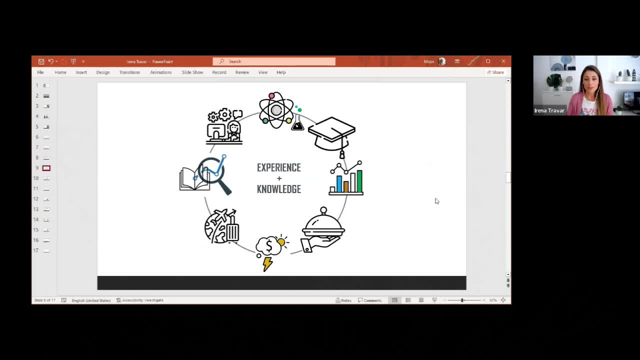 projects that I did. So when we put this together, your experience and your, your knowledge, so you cannot look at them separately. They they are, they need to be, to be combined. So from both of them you will learn a lot of things and you need, you will be able to put in. 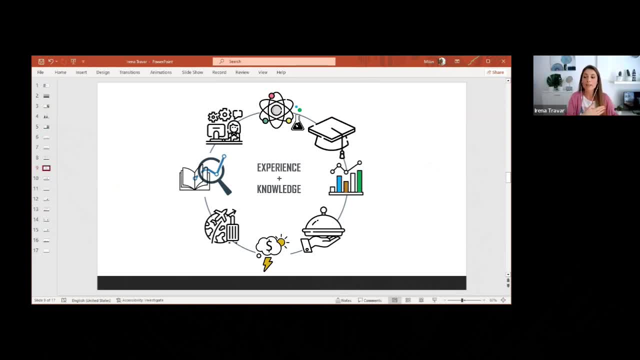 practice what, what you did in your jobs, and your the knowledge that you that you gained. So that is why it is important to accept challenges. Don't, for example, if you receive a job offer and you say, oh, I'm not able to do this. 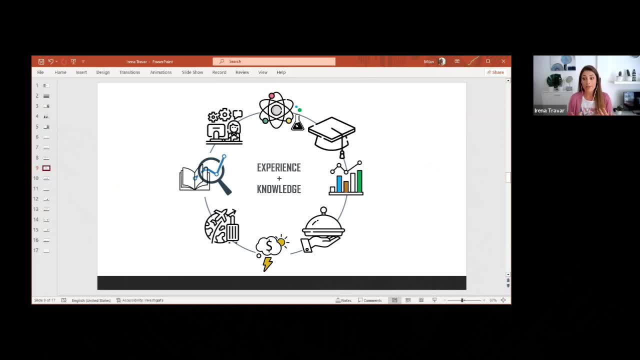 Okay, Everything, Everything you can learn. So just tell yourself, everything really can be, can be learned. I did so many, so many different things. I had different job positions, different countries, And now I work, for example, with with the whole world, When I, when I work remotely. 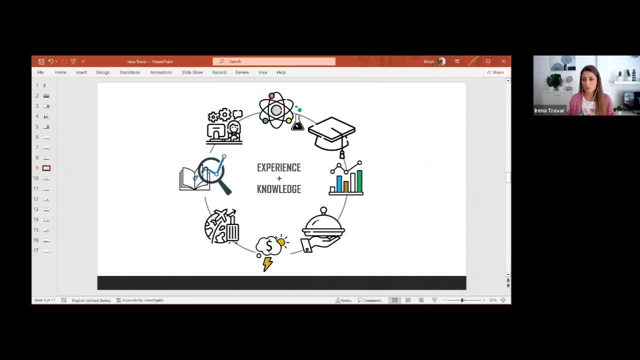 I had students from the U S, from Canada, from Australia. So when they, when, when they text me, when they send me a message that they need, for example, help with supervising them in while obtaining they are maybe masters or PhD studies. 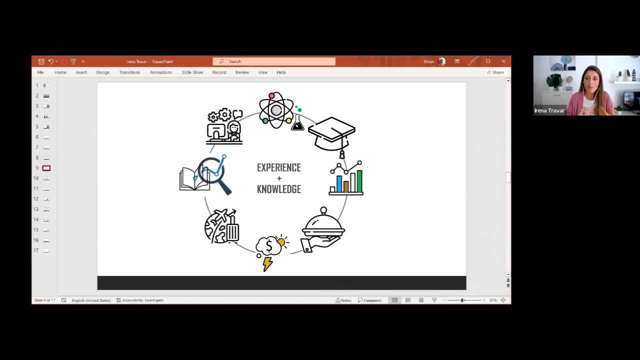 Actually I, at the moment I don't know what I'm going exactly to do, but, okay, I start communication with with them And finally we we find the same, the same language. So that is where your experience is really valuable and as well your knowledge. 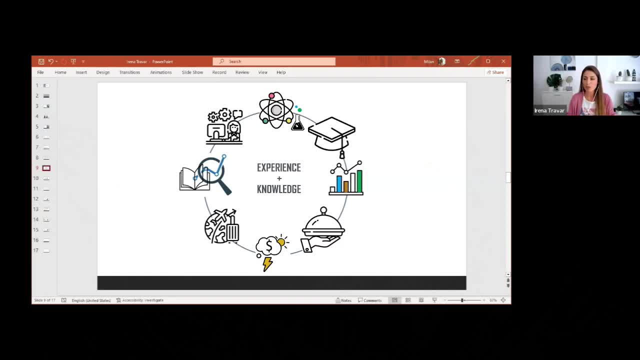 Sometimes people will tell you maybe why are you doing that? You don't need that. Okay, Don't, don't listen to it. Everything that you, that you do- Okay, If you do really, you will have some benefits in in the future. 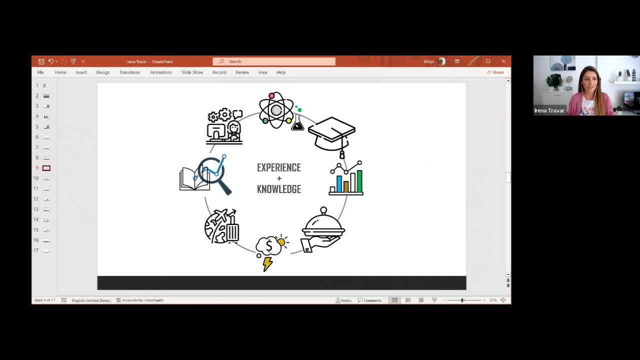 So don't think that you are wasting your time with your studies or doing some job That's not so well paid- paid. If you don't have another opportunity, Okay, You will do that, The job that's not so so well, well paid. but you will gain experience and then you 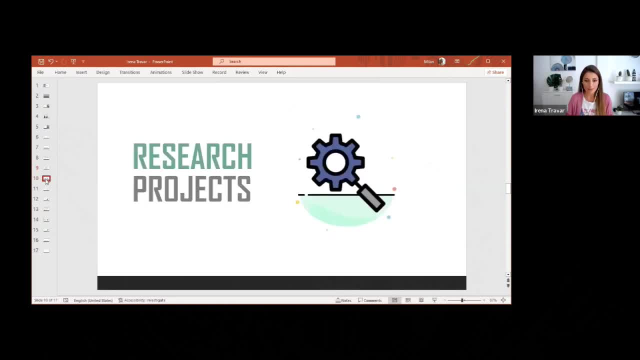 will be able to find a better job, for example. So here I would like to mention some of All my research projects, that that I did, and I also would like to emphasize that all my research projects that I've done, I've, I've, I've been doing them like at the same. 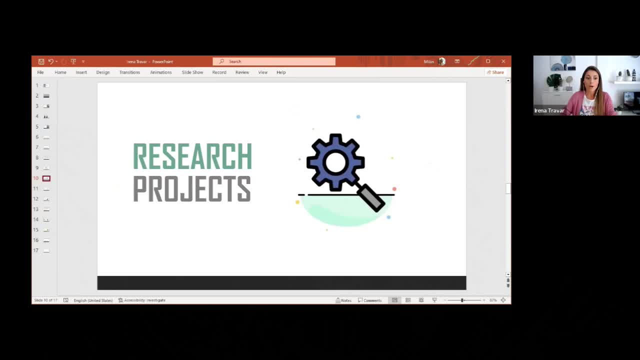 time with while working for or another companies, or now working remotely. So that is, for example, I. I cannot now afford to be dedicated a hundred percent, Okay, Okay To my research projects, but I always have them because that's something that that's. 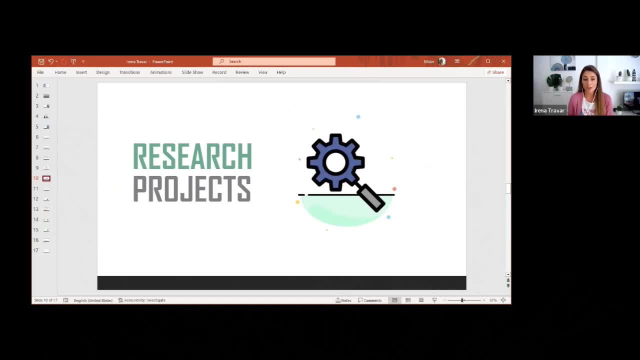 really interesting for me. That's really my passion, And I really have a lot of people who tell me: why are you wasting your time? Go to the beach, but you have beach during the winter. Okay, I will go on Sunday, but from Monday to Friday I want to be dedicated to, to, to this. 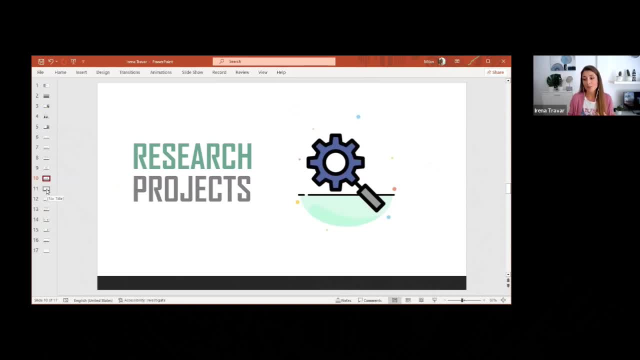 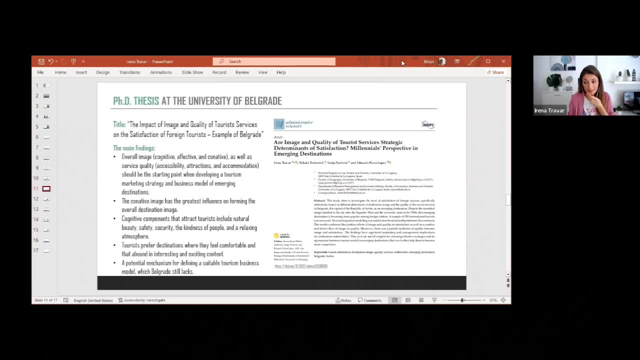 So, actually, uh, that is uh just you need to be, to be persistent and really you will. you will see the benefits Uh, the my PhD thesis, uh that I, uh that I did- is from the university of Belgrade, and 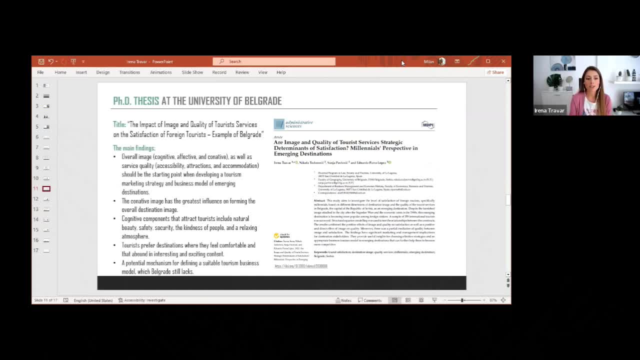 it's the impact of image and quality of tourist services on the satisfaction of foreign tourists. example of Belgrade. So I mentioned you some interesting facts about about Belgrade and about Serbia, And the idea for um uh for this topic came to me when I was uh working as a tour guide. 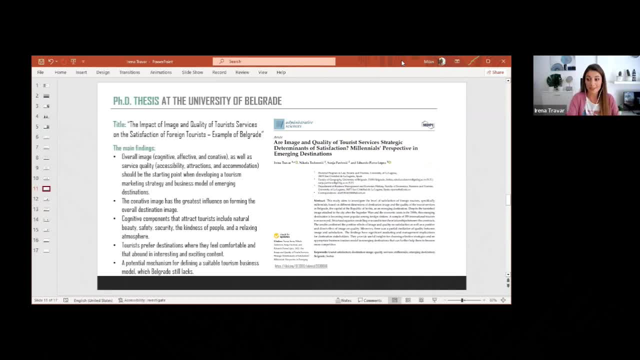 So actually that is what I wanted to tell you: That experience that you, that you have, is really valuable for you later, even though at that moment you don't see why, maybe it is valuable. but after a couple of years, after a couple of months, maybe you will. you will really see that that it was. it was valuable. 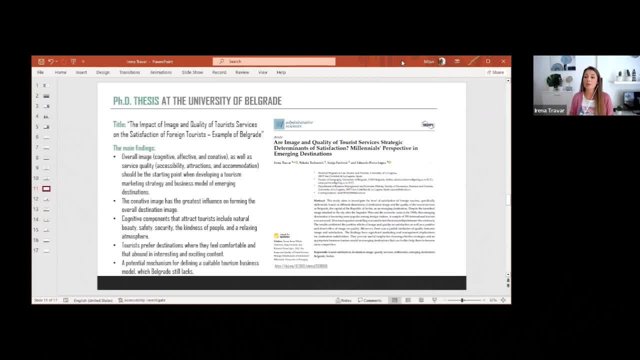 So actually I realized that, uh, tourists that come to Serbia, uh are some tourists who traveled a lot, for example, who visited Spain, France, who went to the U? S, to even some China, Australia, So and then they said: okay, I can now go to to Serbia. It's small country And okay. I visited so many countries. Why people don't don't come, uh, why not many people come? come to Serbia, Maybe. we have in Belgrade 2 million tourists yearly. That's actually nothing compared to other big cities in uh in Europe. 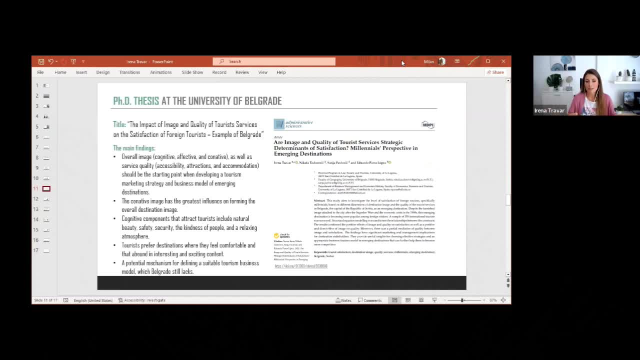 Uh, and 1 million are international tourists, 1 million are domestic Tourists. So you see that these are not some some numbers that we we should be really satisfied compared to the destination that uh, that we have in something that that we can offer. 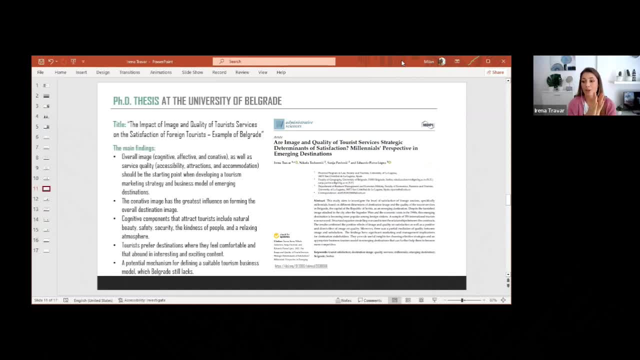 So I had uh one, a couple from uh from the U S. uh, they came to my tour and I was guiding them. It was the underground tour of Belgrade And I was talking to them. Uh, I asked them, oh, why you came to to to Belgrade? 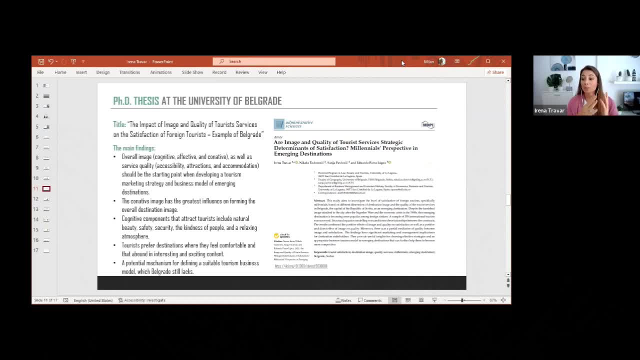 Why you came to Serbia. And they said it said to me: oh, because we are explorers, we want to explore new destinations. But when we told our friends from uh, from the U? S, that we were going to survey, they said: oh, you must be crazy. 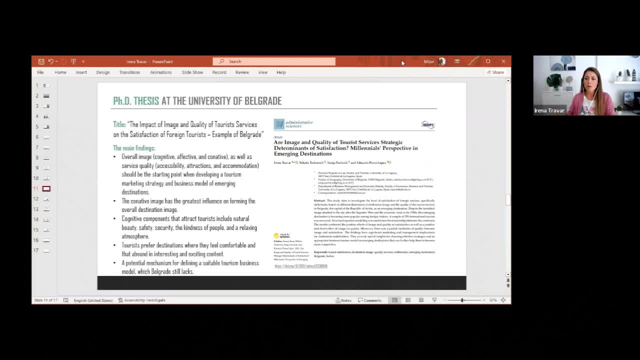 Don't go there. It's a destination There is. there is a war, You don't. you cannot see anything interesting there, but actually the information that we have in in in the media, uh, I think that 90% is is not true. 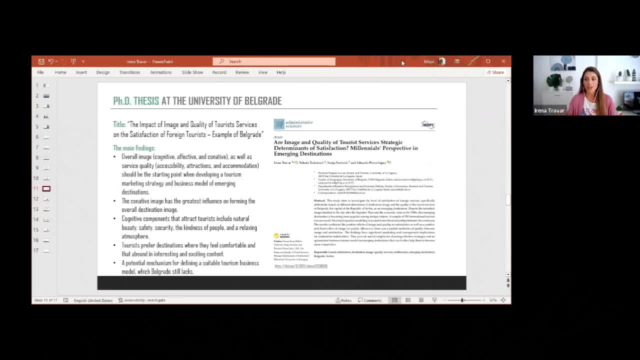 Really You need to, You need to investigate on yourself. So when somebody tells you, don't do this because they, they know, they know better, So investigate on yourself. People told me: oh, Singapore, you will not be able to receive an offer from from Singapore. 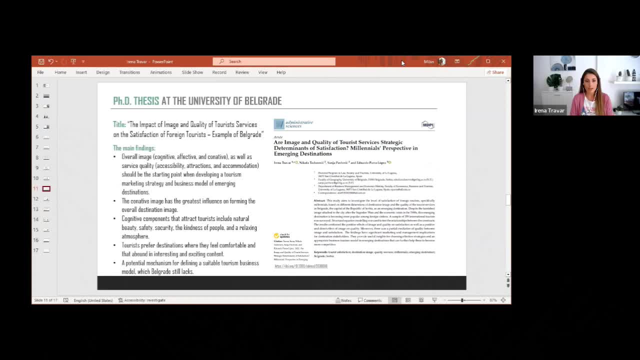 Imagine me sitting at my room sending 400 emails and people tell me: what are you doing? Come and enjoy with us. Let's go to some bar to drink something. No, I stayed at home and I really had my goal in front of in front of me. 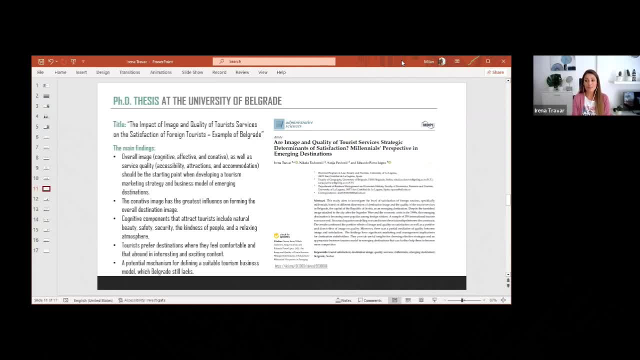 So actually, that's what? What? uh, uh, their, their friends told them that they were, they were crazy to go to Serbia. but they investigated, They, uh, they did their own research and they, they came to Serbia. 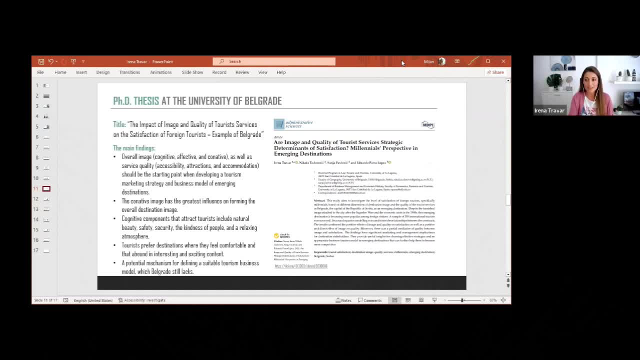 And of course, they were very satisfied, because people who come, who visit Serbia, Belgrade, really say that we are really generous people And uh, uh, and at the end they are satisfied. So that is how my idea, uh, how I got to the idea on on what to do. 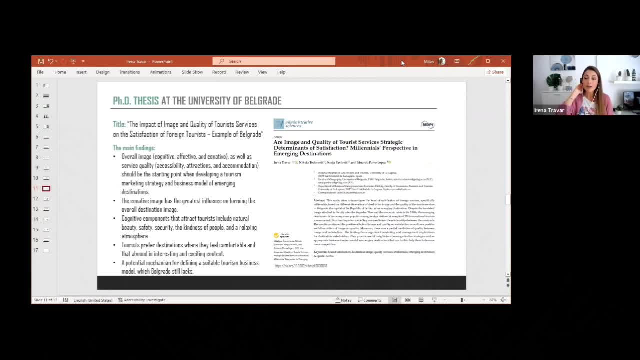 I wanted to investigate the image and quality of tourist services and how it influences tourist Satisfaction. Uh, this C? here is a paper that I published. It's um is part of my PhD dissertation that I published uh last year. 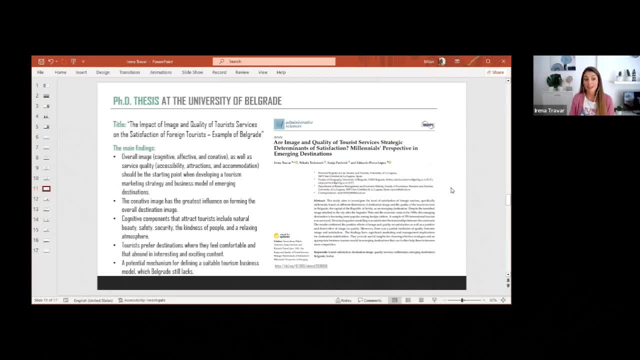 And uh, here I put some of the main of the main findings that actually image and service quality really influence um satisfaction and that, uh, that, uh, my goal was to uh to have a base like to create a business model of um a future development of Belgrade as a. 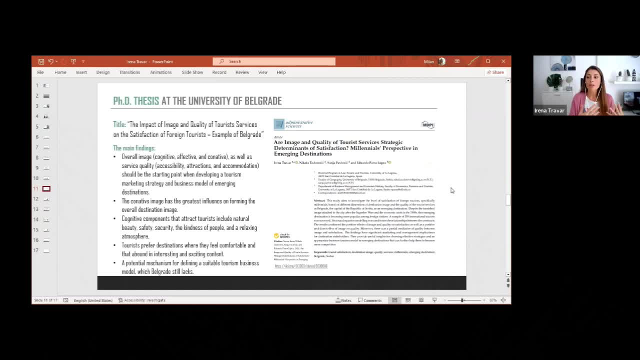 A tourist uh destination because uh actually there is not a tourism business uh model for for the future uh period, And I also found that tourists, for example, are very interested in natural beauty, safety, security. 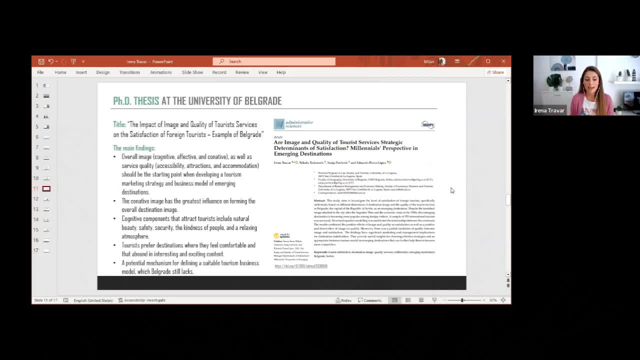 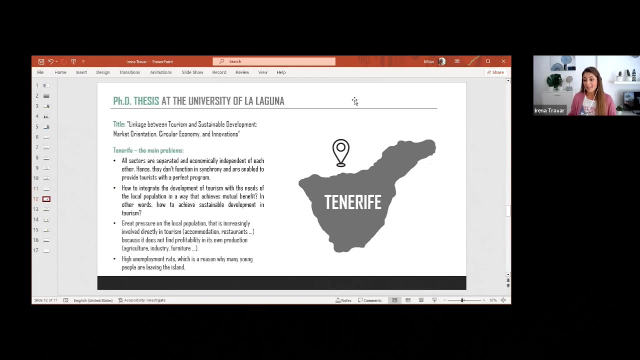 They like generosity, kindness of people, They like that relaxing atmosphere. So these, these were really uh important findings for um, for the developing of uh um of suitable business model. Well, this is my, My second uh uh PhD. 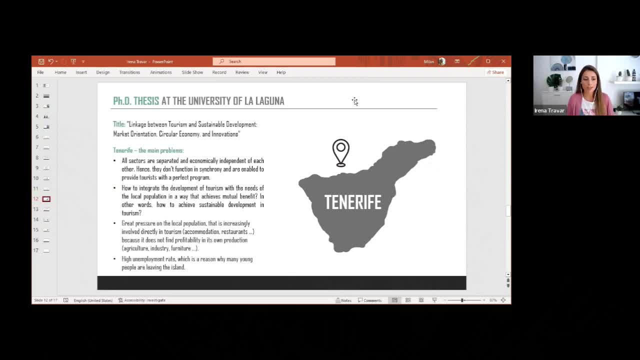 So maybe you can now think, oh, why she's doing? why she's doing two PhD uh thesis? Um, so what? what happened? I came to Spain. I- at that moment it was three and a half years ago. 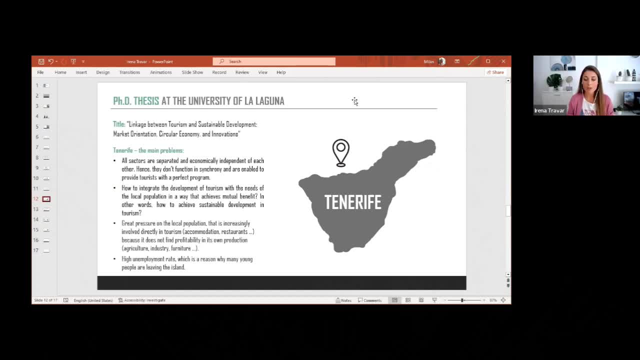 I didn't finish my thesis at the university of Belgrade because I couldn't publish paper. Uh, so what happened? Journals did not accepted papers that I was sent. I was sending and sending with my professors from the university of Belgrade and I said, okay, nevermind, let's leave it. 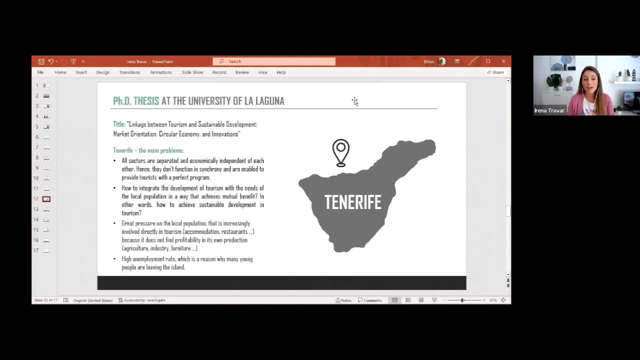 Uh, I will start my career here. I want to stay in Spain and I enrolled to the PhD uh program at the university of La Laguna. I really liked it. I liked the group that I'm working with, my team and uh and everything, and how supportable we are to for to um uh, each other's uh and what. what happened. 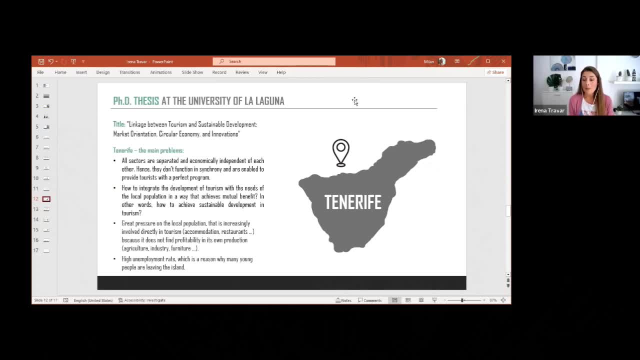 I enrolled to the university Uh of La Laguna in in Tenerife and I received again another email. So look at this: another email that my paper was going to be published and that now I can uh defend my PhD thesis at the university of Belgrade. 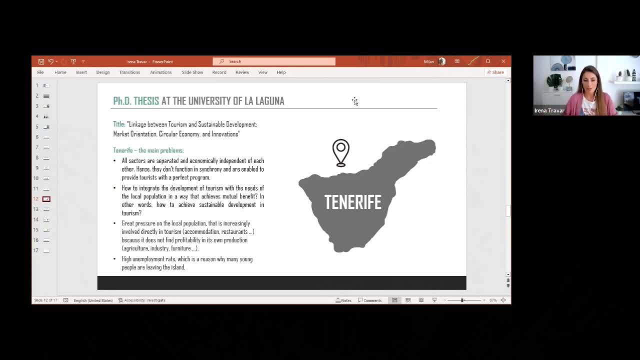 So what to do here? I already was enrolled. I like sustainability, I like this concept. I'm I'm really amazed by Tenerife as a tourist destination And, on the other hand, I have another PhD thesis waiting For me. 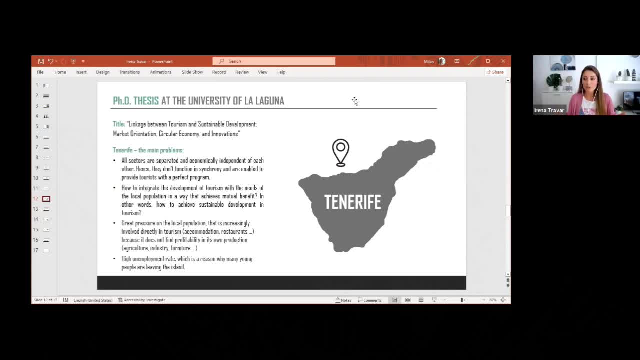 So I said, okay, let's dedicate this two or three months to finish this for Serbia, And then I'll continue here in Spain, And that is that is what I did. Believe me that, uh, only my parents believed in in me, in, in in that period of time. 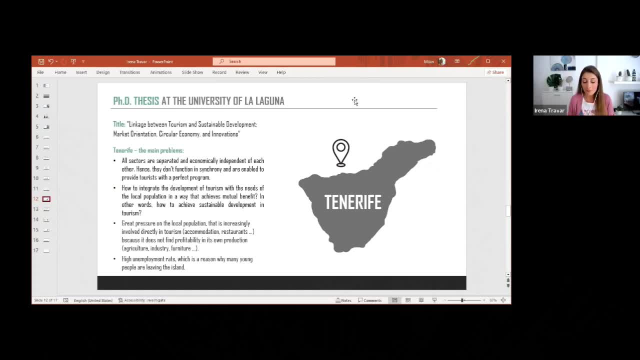 And I'm very grateful for for for that, that they supported me. First of all, they supported me financially because to to finish a PhD, you really need to be dedicated. So this two or three months while I was um. 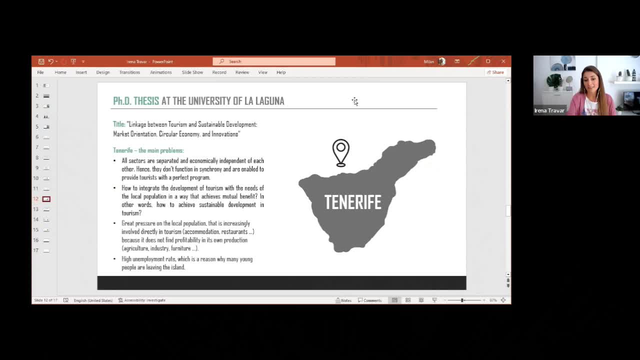 Writing everything, all the findings, uh that that I find for for my empirical research. So they uh, uh, they supported me, but of course they, they told me, okay, just now, and then continue with your studies, work, whatever, that's it from us. 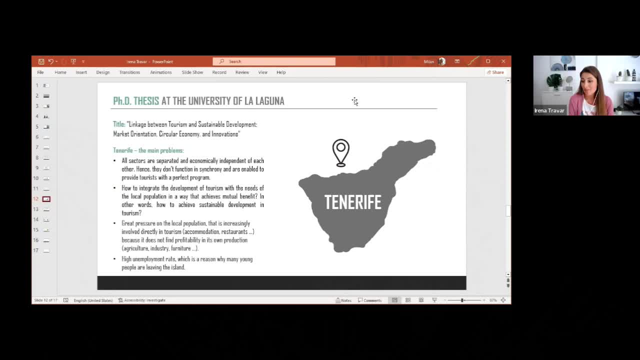 And then I finished uh, um, of course. now I'm PhD uh in in geosciences, in uh in in tourism, from the university of Belgrade, And I'm also doing my second PhD here at the university of La. 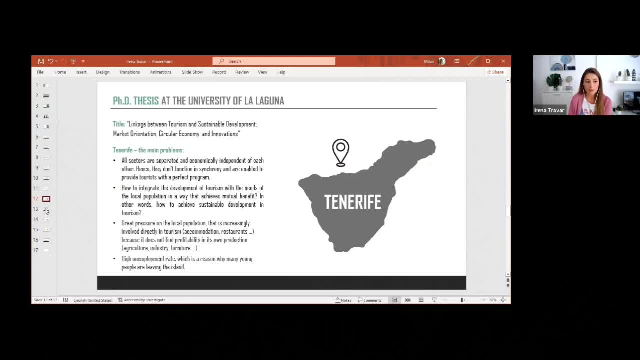 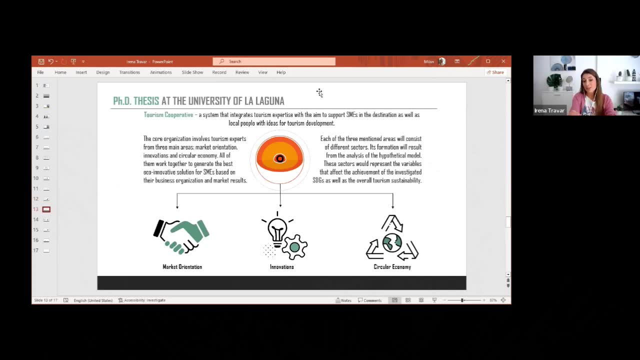 La Laguna, where um I'm also involved in some projects, and here I would like to uh to present you uh my my idea actually about sustainability. Uh, I want to investigate market orientation, innovations and circular economy and how uh they are related, how they influence uh sustainability. 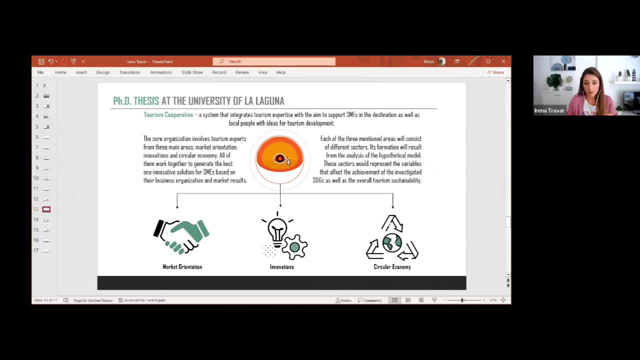 So my idea came from the earth: that you can see, that you can see here and the core. uh, that is my idea. My Final goal actually is, uh, to create a tourism co-operative, that is, a system that integrates tourism expertise with the aim to support small and medium enterprises, because you know now that I had um a lot of experience with small and medium enterprises- I was working as a tour guide. 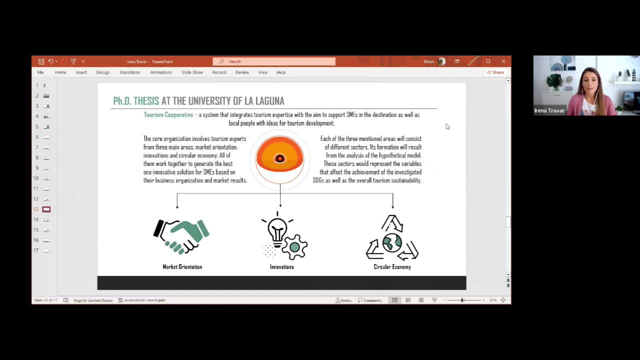 So, actually, I was a kind of entrepreneur and, uh, I want also local people to be included because, um, for sustainability, it is important that uh, we have A lot of support. Uh, so, uh, that is um, uh, something that I'm currently uh investigating, so I cannot give you more, uh more information about about this project, because everything is in uh in the process now. 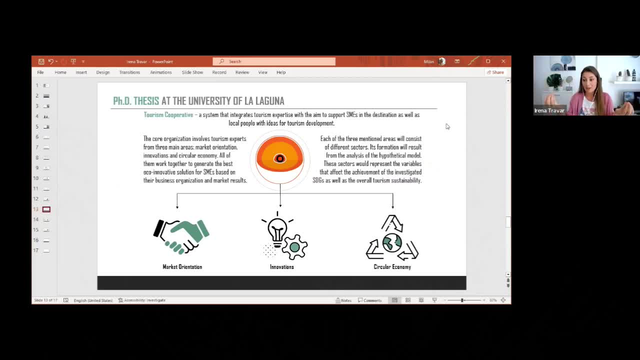 And, as I told you, I have my idea and I have my, my goal. So now I'm in this process, uh working on it, to uh, uh, to finally, if it uh, if it's possible to, to create. 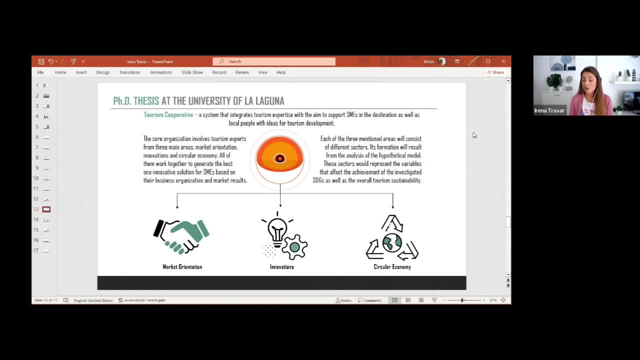 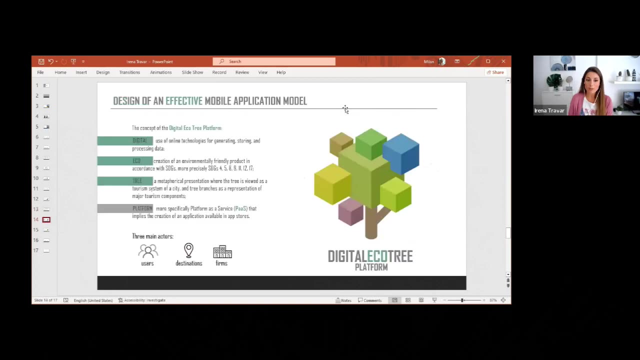 A pilot project here in in Tenerife for for tourism cooperative, where I would like to help small and medium enterprises to be more sustainable. So to work according to sustainability uh principles. And the last uh thing that I wanted to mention is my another project here at the university of La Laguna. 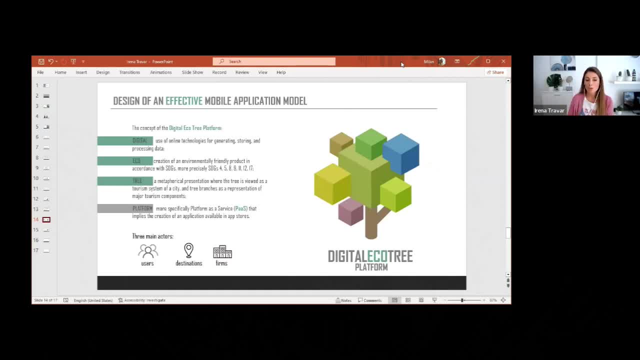 It is design of an effective mobile application model. So, even though I'm not a technology expert- Again, That's not what I told you- I have the idea and we, we have- um, we will find another, uh, researchers- that that will help us to put in practice this mobile application model. 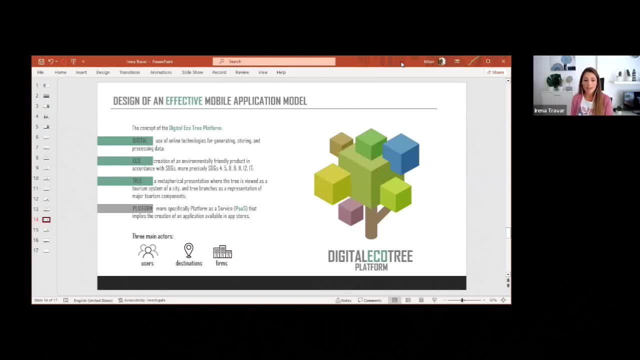 It's a digital eco trade uh platform. uh, that, uh. I want to, for example, to Uh to help all tourists who visit certain destination to have one useful app where they will be able to find all the information. 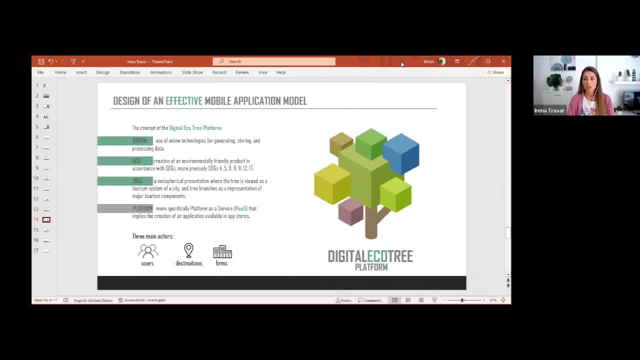 destination, for example, to see real-time information. if they want to visit some attraction to see in the app, oh, how long i need to wait to enter that, that attraction, because you know that sometimes, uh, you want maybe, uh, to visit sagrada familia in barcelona and you need to wait. i don't. 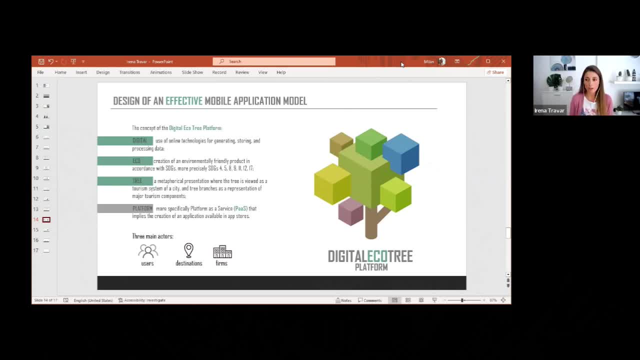 know two hours to enter and then you say, oh, i don't want to wait, let's see what attraction i can, i can visit where i don't need to wait so long. so that is one of the of the ideas that i have. uh, of course, i still don't know how to put in practice. and i don't need to know, i'm not a. 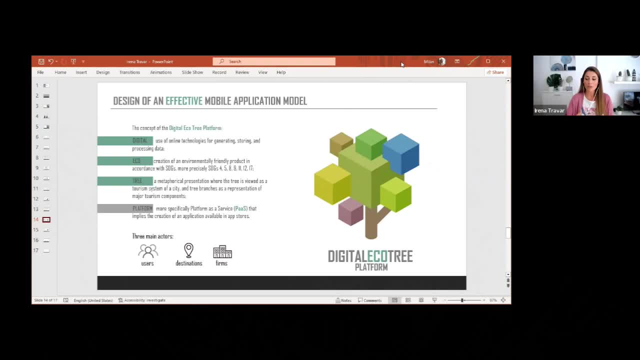 technology expert but of course, it's important that you work in a group, that you work in a team and i think, as as students, you i'm sure you have many, many projects where you work as a team, so everyone can contribute. so it's important that you cannot know. 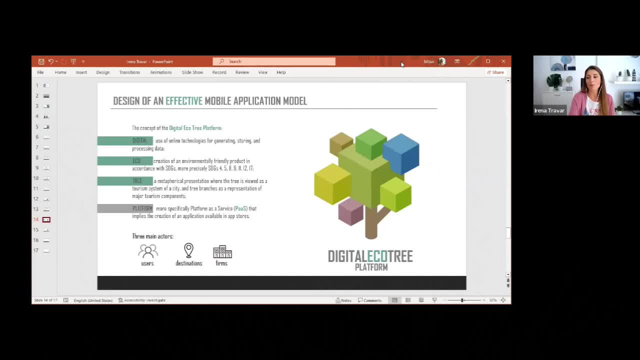 everything, but you will find people who know, you will find people who can uh, who can uh help you. so that is this, um, this project about digital echo tree platform: uh, so actually to use the online technologies again to work according to the principles of sustainability, which uh is actually. 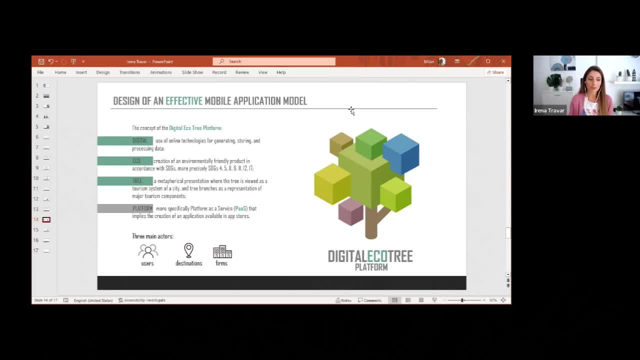 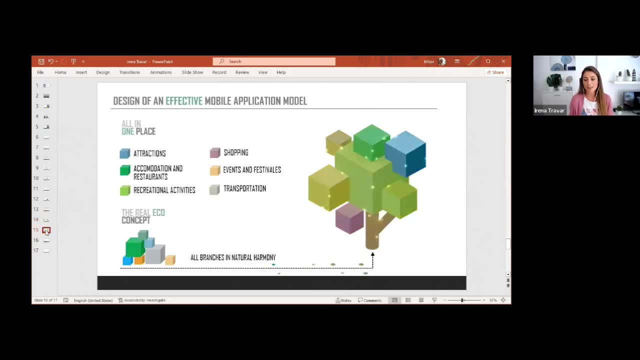 my, something that i'm i'm really interested in and i'm working for my uh, for my phd thesis, here. so this is: i wanted to say that we had a participant who wants to ask a question. akita salim, if you're able to, let me see if i can find you. 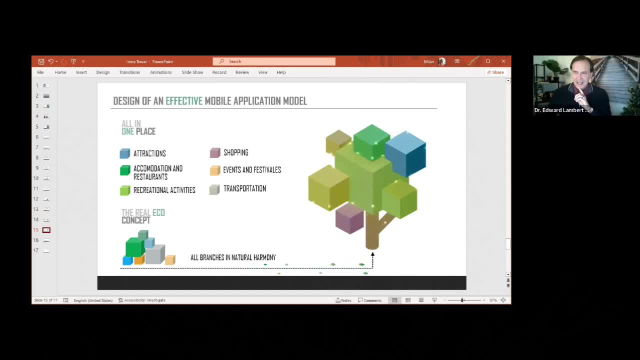 yeah, he had his hand up for a long time. i see him. i see him there, you do. yes, can you ask to unmute the microphone? yes, akita, you have a question for you. you had your camera on your hand up for a long time, um, so now is your time. can you hear us? 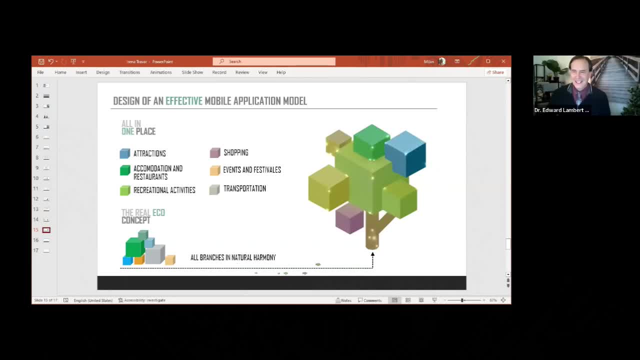 akita. you know i cannot find him in the list there. yes, i'm here, hi akita. yes, please, um, you wanted to share something with uh, with irina, our presenter. yes, yes, i just want to ask you a question. of course that, yes, i just want to ask the question to irina. 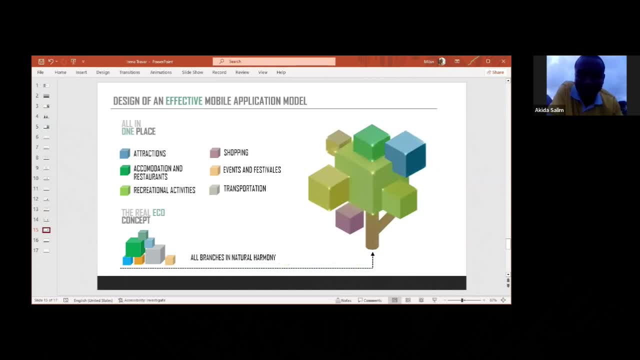 hello. hello, yes, you can ask. okay, yeah, my question is how the tourism can bring the positive significance toward the religious issues. okay, can you, can you specify it's? it's very broad, broad topic. what kind of uh of religious issues, any example? or right, maybe in christianity, the changes because those tourists, when they 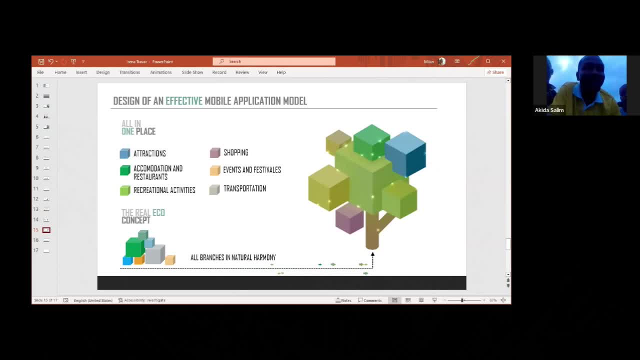 are coming from their home countries and the changes they can bring to the, to another country they go for tourism activities, so something like that. the issue of cultural changes, behavioral and so forth, yes, okay, yeah, i will, uh, i will answer, i think i uh, i know what, what. 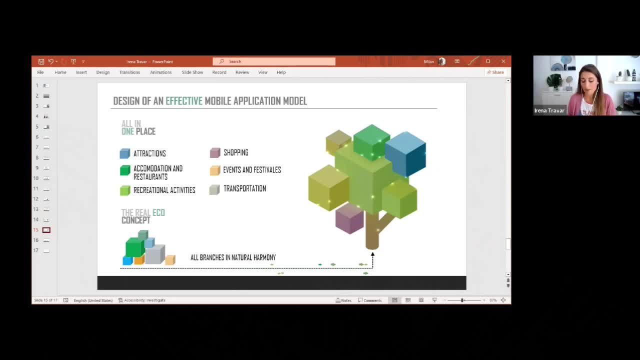 actually wanted to ask me. so, uh, when i answer you can, you can ask some some sub questions. uh, so, actually, uh, of course, when, when tourists travel, we there are a lot of problems for, uh, local, um, for local people, because that is the problem of mass tourism. you have um, for example, 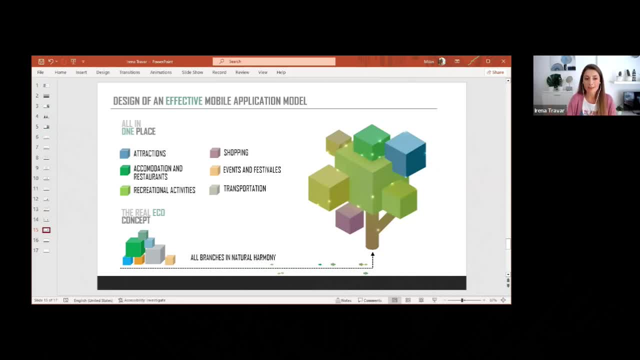 the number of tourists that come to one destination and they- um, sometimes they destroy completely the, uh, the, the local tradition, the local life, because they have such a big impact. uh, so that is why, uh, also, i'm- um, i'm interested in sustainable tourism so that tourists who come 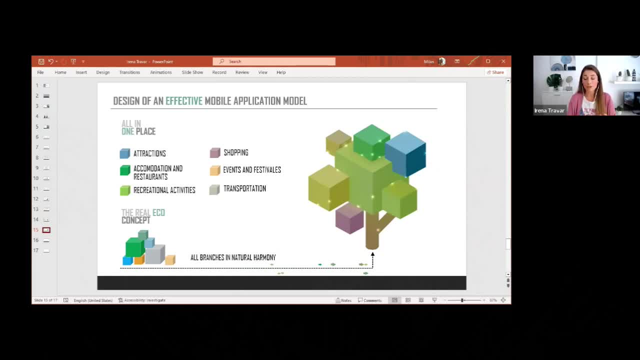 that they don't disturb the local life, even though it is a religion, it is tradition, it is culture, it is just their, their life. so when, um when, when tourists come, when tourists visit some country or some some destination, uh, so that they, um, they actually accept everything from the locals. 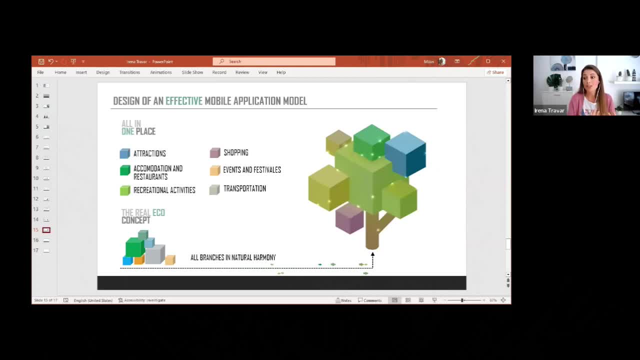 they can be part of their life, but not to disturb the local life. uh, it is something that, for example, uh need to be done by local governments. uh, we alone are not uh able. we can raise our voice, but, um, uh, we are not able to to change that. uh, so actually, 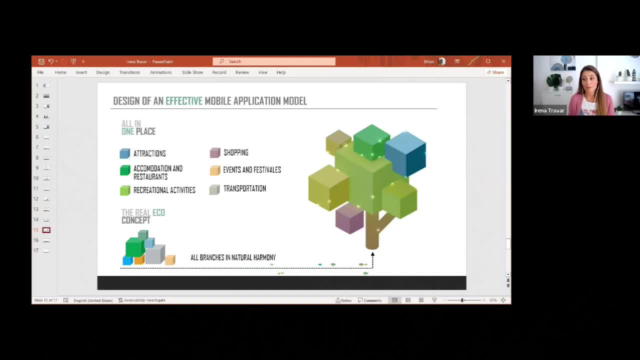 for example, i can, uh, i can tell you examples what here in tenerife, uh, we are doing. we have, for example, some parts where so many tourists come and these places become so touristic, uh, and you know, you even cannot see locals, and locals go to their, to their towns, where they feel. 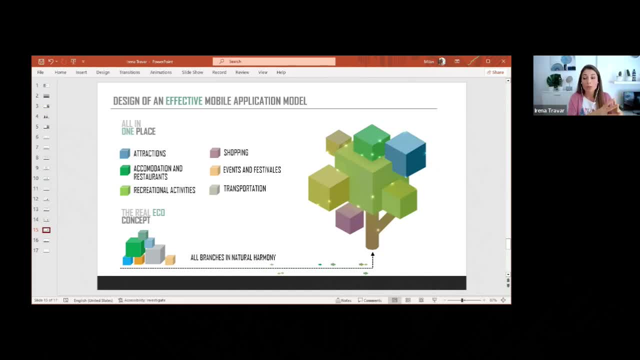 where they feel safe. uh, so actually we need to limit the number of tourists. it is the question for for the government. uh, and then from from that point, we can decide, okay, where tourists can go, what attractions they can visit. okay, this is a museum, so maybe- i don't know- 200 people a day. 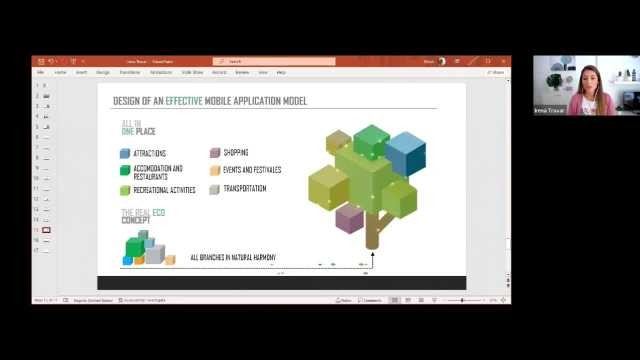 can visit that, that attraction. so, with certain limitations, we can help local people to have benefits from tourists. okay and uh, not to to disturb them or or to to destroy their, uh, their regular life. so that is why, uh, for example, also in my phd thesis at the university of laguna, i want to include local people. i want. 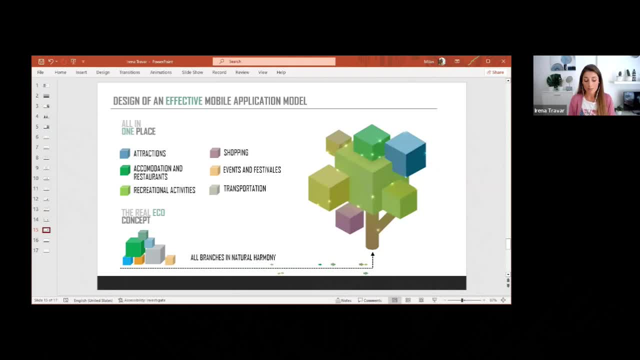 to help small and medium enterprises that are actually, uh, the biggest number of um of firms in tourism are small and medium enterprises. they usually don't have financial resources to work, uh like in accordance with sustainability, uh concepts, and i want also to include local people, so everybody can raise voice and then we can find a solution. so, actually it is, it is something. 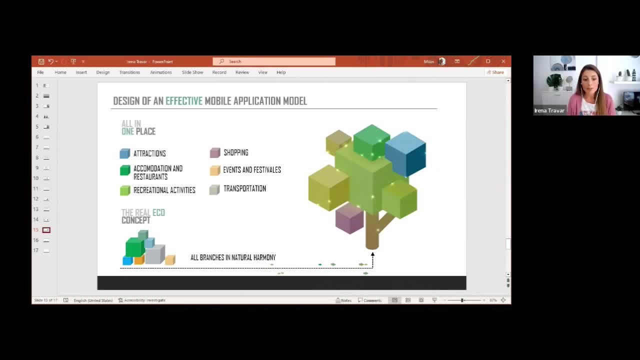 uh, it is on the local government and i know sometimes the process is very slow, uh, but uh. but actually, if you have, for example, if you're not satisfied what is happening at your um, at your home city, you can always have some organization with uh, with a group of people. 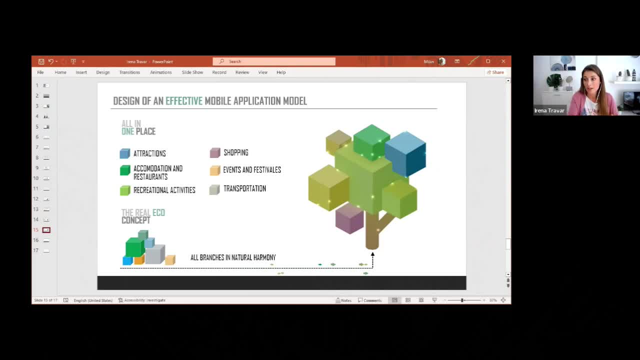 that you share the same ideas and and present them as a solution. so actually, that is no, some universal solution from the problem. each destination is different. uh, so, uh, you, you, really, if you ask me for some particular destination, maybe for for your city, uh, that means that 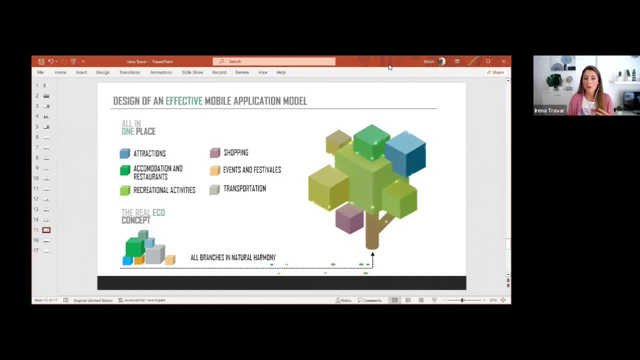 uh, you need to to have all the factors in mind to to well find a way or to to present them to to the government, who that will that will decide on on future actions. but actually, uh, united nations is is working on that and that is why uh 17 sustainability goals uh were developed. uh, actually to help. 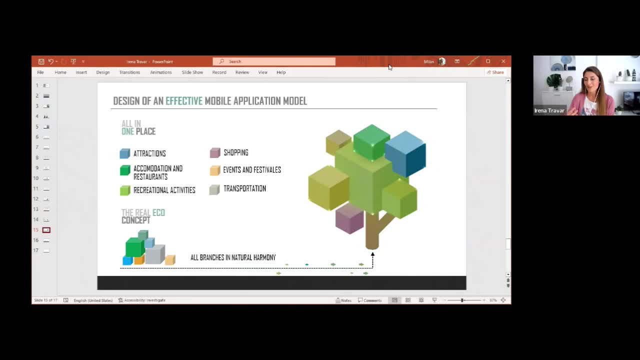 all local, local people because, you know, attraction for tourists are local people. it is local life. me a tourist, for example, when i, as a tourist, when i, when i travel, i want to see how local people live, you know, but i don't want to be the one who is the loudest, who, who, who will disturb them? uh, so we need. 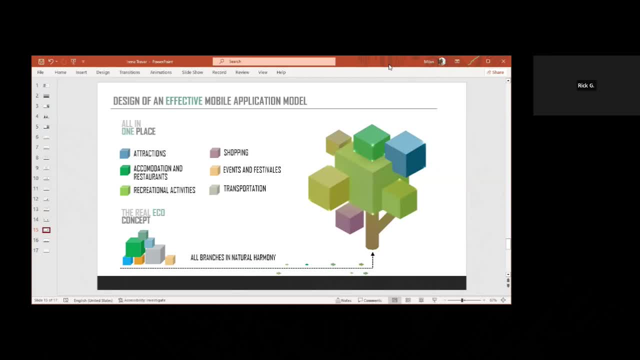 to find the balance. thank you, irina. yeah, i was. i was just gonna say that, uh, yes, i agree with everything you're saying and, uh, akita's concern, i think, is very valid and we just have to understand that people are in different stages of evolution in their life. 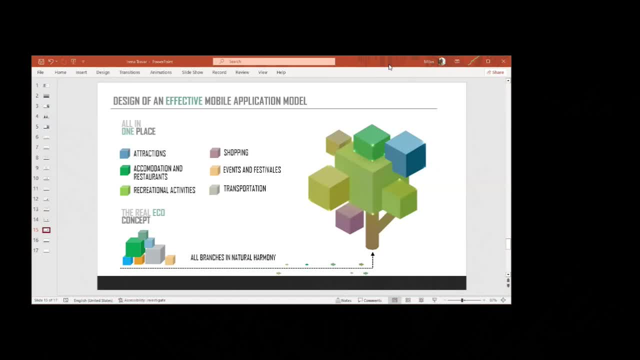 you know, some people understand and respect those things. some people are still young in that regard and they may do something that to us appears disrespectful, but we have to look at that person with love and understanding. if we start with love and understanding, i think- uh, it will be a much. 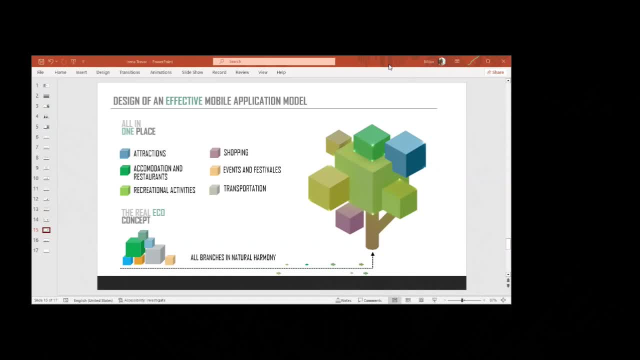 better interaction, whether you're a local or a tourist, because your energy will be towards helping what might be encroaching on your values, whether it's of your city or your religion, but if we understand that we're both here on a mission of evolution and growth. 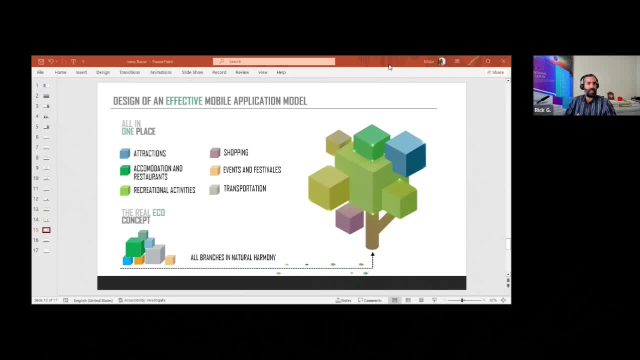 i think if we start from there, all of the interactions that we have can be positive. and, irina, you mentioned the unesco 2030 goals. we actually have something called the aiu pledge, so all of our students, at some point in the program, pledge to contribute uh towards achieving 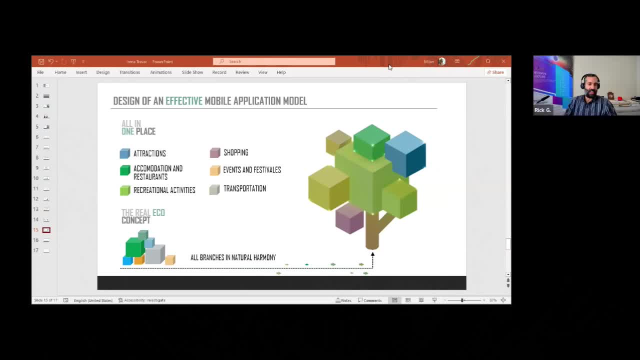 those goals, because governments can't do it by themselves. they need participation from all of the global citizens and we're all empowered to contribute in some way. to think: what are my unique skills? how can i do something uh towards, help, uh towards one of those goals? uh, so thank you so much for bringing that up. that's, that's, uh, that's excellent. you're the. 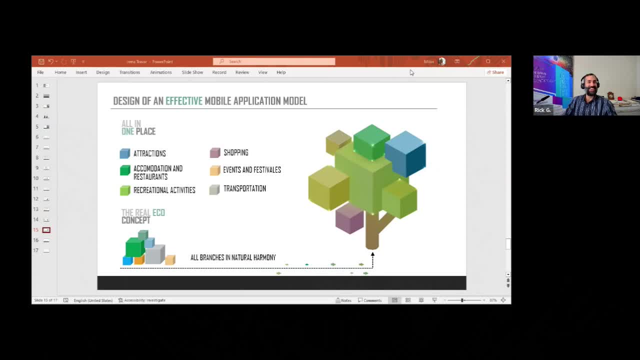 first presenter that's brought up the 2030 goals, so thank you so much. thank you, dr lambert. uh, go ahead. thank you, akita, for your excellent questions. go ahead and continue with your presentation. okay, of course, i'm i'm almost done, so actually you can think about your, your questions and and. 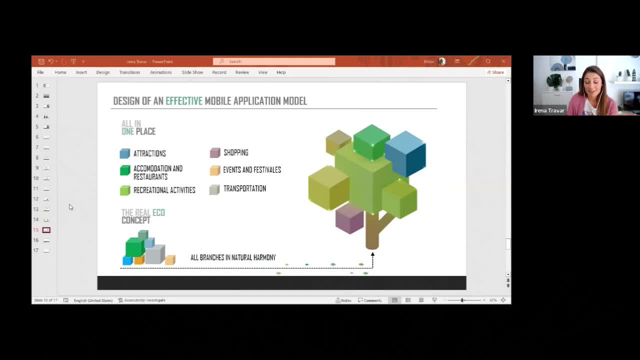 we can have a discussion. uh, so well, what i also uh mentioned here, this is just um, my um, the model of of effective mobile application, uh model, where i found that uh, for example, what is the most, the most important for tourists in one destination are this, um, this six uh things. 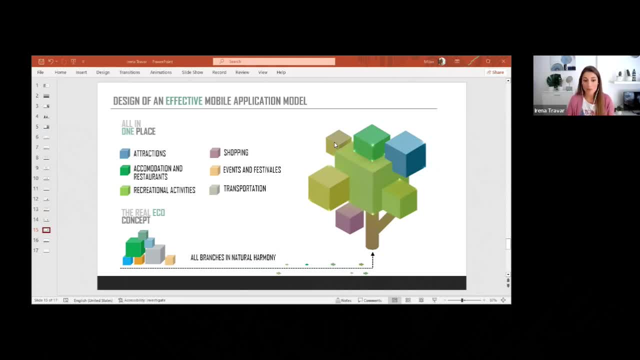 these are attractions, accommodation, restaurants, recreational activities, shopping, events and festivals and transportation. so actually i would like to include all of this in one mobile application and, uh, to work with, um, with firms that, uh, that actually are sustainable, uh, so that is. that was everything about that that i wanted to say. 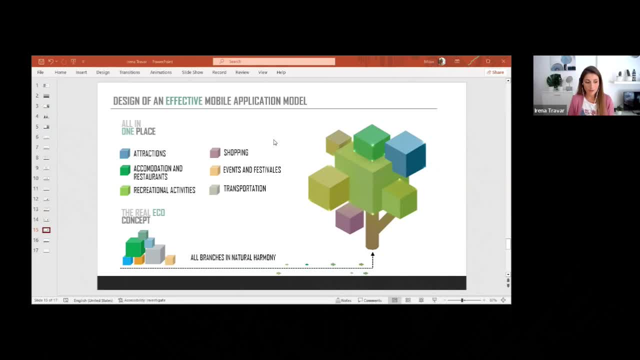 to to present you so actually to know what i'm, what, what i i've been doing and what i'm dedicated to. so, of course, if you have more questions related to the tourism or some some other questions about what i mentioned, or actually you want to ask something else, you are free to to do it. 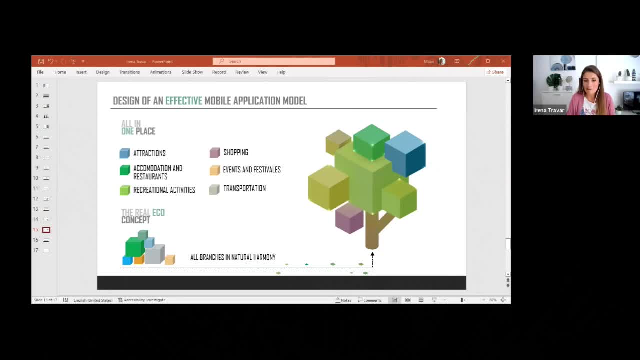 so do we have more questions? yes, it looks like we do. we have uh questions from a couple of participants. there's one that was written down. uh, let me read that one. um, it was uh, basically, how, how could they uh, how could they uh utilize the potential of the local? 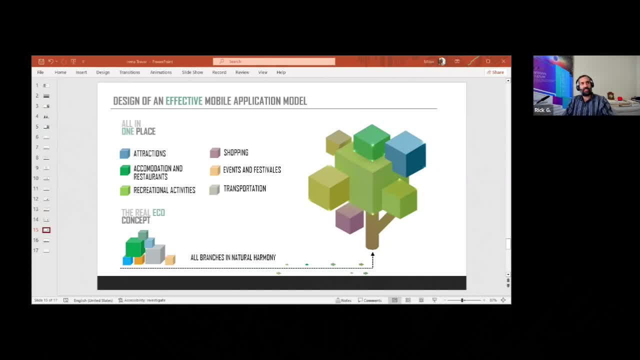 tourism. in other words, what are some tools or what are some specific actions that you recommend for someone who may want to offer services and tourism in their local city? i don't know if there's some tools or some training, i mean. i mean, i don't know if you typically maybe would. 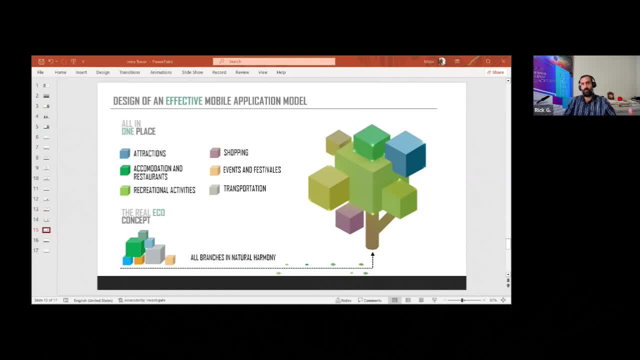 start off showing, uh, planning a trip for a family or a friend and kind of getting experience on- hey, how was your experience? what could have been better? and then maybe offer your your services. so that was a question from one of our students, um, from earlier in the presentation. i don't know. 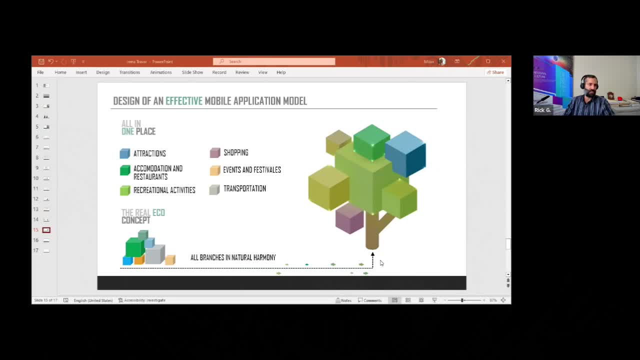 if you have any specific tools or suggestions for that. uh, well, of course. that means if you want to start developing tourism, or to you want to start working as an entrepreneur in in your in, in your local city. that is correct. okay, yes, of course. uh, well, uh, there are many uh. 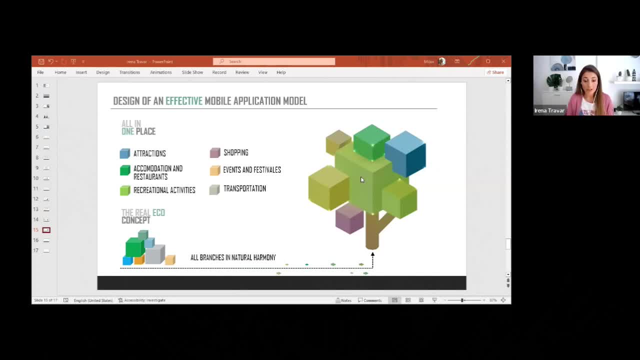 online uh webinars that you can, that you can attend. some of them are free, some of them you need uh, you need to pay and uh, it depends really where you live. i can tell you now for for spain, for tenerife, here, for example: um, like, every municipality organizes some kind of trainings for 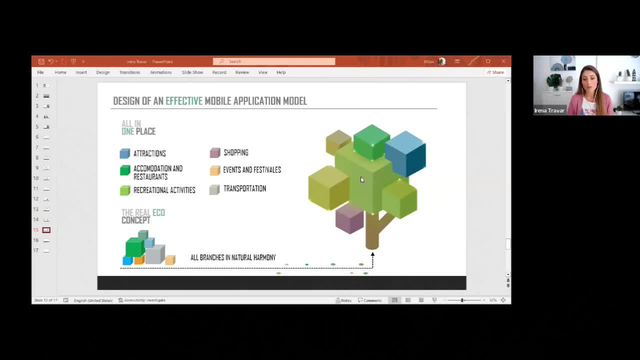 local people who want to start working as entrepreneurs. so there you can maybe learn how to uh, how to have a facebook page, instagram page. uh, that is efficient, so that will attract tourists. it's not only to have it, it's important to know how to track it. for example, what pictures to 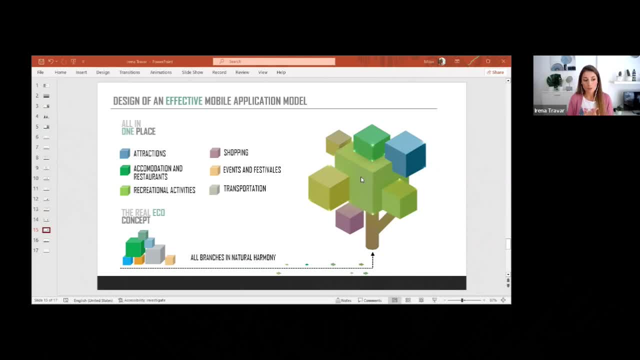 upload, what time to upload uh, how to uh how to reach more followers. so you can find a lot, of, a lot of answers on the internet. but, of course, if you have a possibility uh to participate in some webinar or some or some training, go ahead uh the. 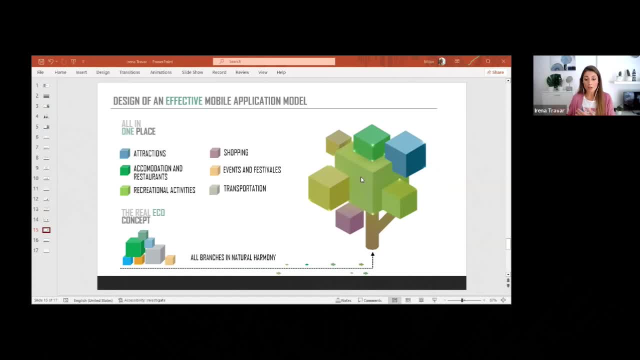 that will be really helpful. and, of course, if you have maybe some accommodation that you want to adapt for tourists, you can. you can use airbnb or booking because, for example, when i lived in singapore so i traveled to indonesia because it's very close to singapore. indonesia is not developed country, it's 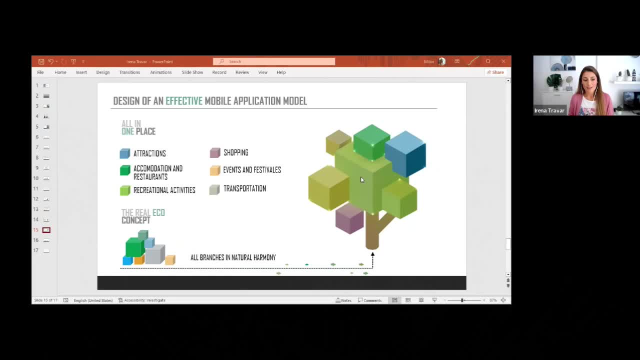 developing country, but actually some islands uh are so small that they even uh don't have roads on the island. they, they, they don't. they don't have cars, they maybe only drive bicycles or motorbikes. but they all have booking. so i find accommodation on booking and then i can, i can. 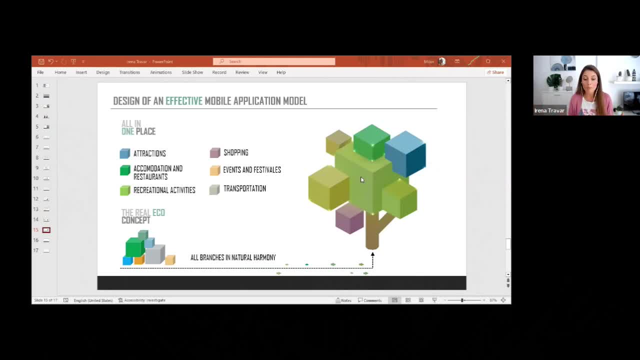 explore the destination. so, where, wherever you live, whatever part of the planet you can, you can use this kind of tools like booking, like airbnb- that that i suggest for the beginning- and always ask people to write a positive review, because reviews are uh something that when you google uh some accommodations, some destinations, that will be something that will 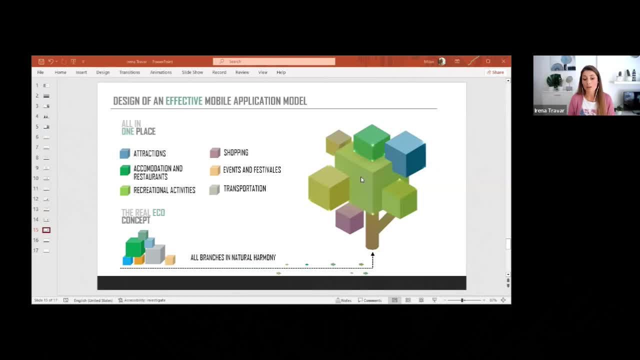 first appear, and if you are ranked high on google, that means that you will receive more, more potential tourists. fantastic, actually. yeah, that is. that is something that now i can just, in a couple of sentences, uh, uh, tell you. but, of course, what, whatever option that you choose will be, will be. 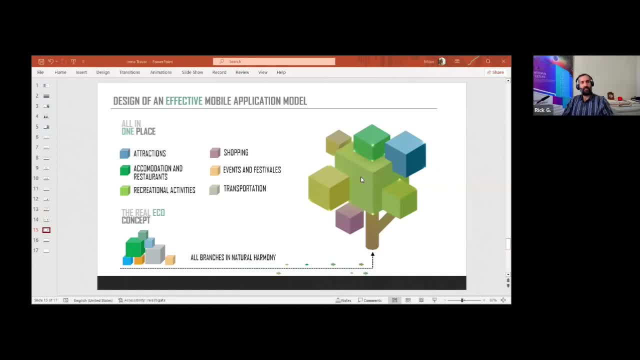 good, fantastic. thank you, irena and uh, we have one more question. uh, we'll see how quick it is from techno spark. uh, techno spark. okay, let's try, emmanuel oru. you have your hand up, emmanuel. you want to comment something or ask a question? 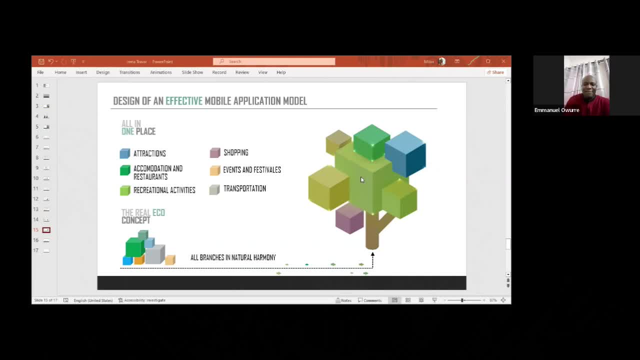 hi, emmanuel, okay, yeah, fine, i've omitted. now, all right, so fine. so, uh, you did mention as a tourist guide that when you have these tourists come into the country and then they go back home satisfied if they see that the people are kind, they are accommodating, they are loving. now what about if there's a gap? maybe 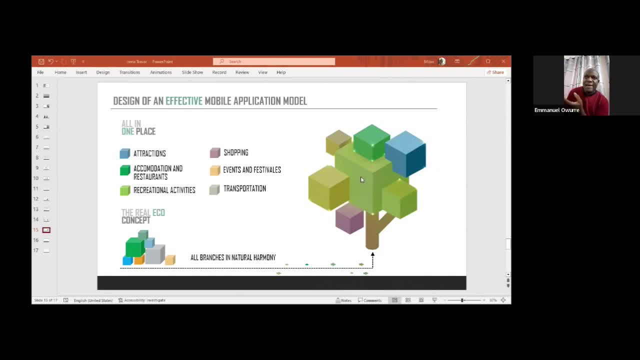 there's a gap in one of those streets that have been identified and your customers are not satisfied because maybe, for example, uh, they are not uh polite and it's not affecting your own business as a, as a guide. so how can you close that gap? because now it's a society trait. 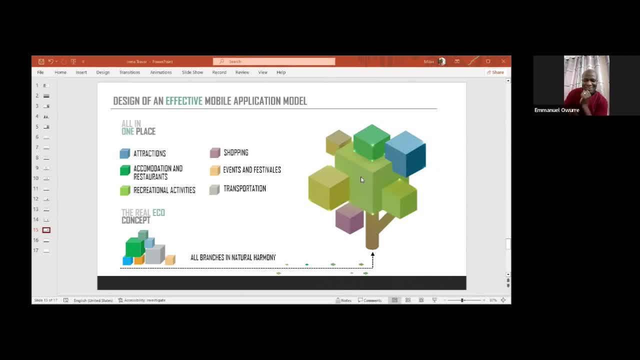 from your own standpoint. how will you address that? so, when i have tourists that are not polite, that is what you wanted to to mention. no, if, uh, the authorities give you a feedback that the, the people are not polite, so you have that now as a gap, it's not affecting your own business as a guide. so 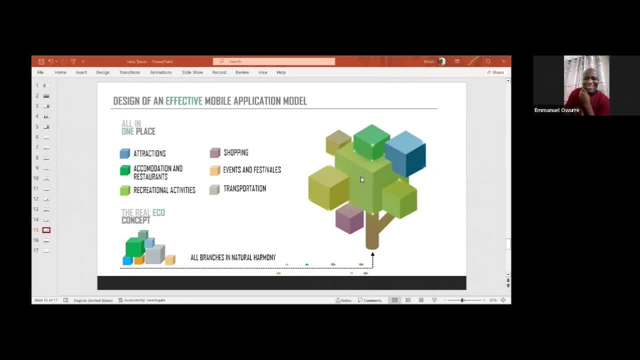 how do you not close this entire traits? okay, so you mean that they live a bad review? yes, well, i always try to to give my best. again what i mentioned: adaptability. i don't guide the same a group of 20 people or 50 people, a group that come from latin america, or 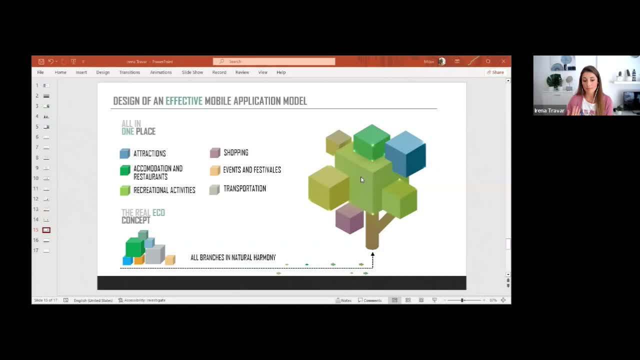 from the us. they all have different interests so i as a as a tour guide, i try at the beginning to just start some informal communication with them to see what they like, if they, if they are interested more in history, okay, i will talk more about history if they want to, if they're interested. 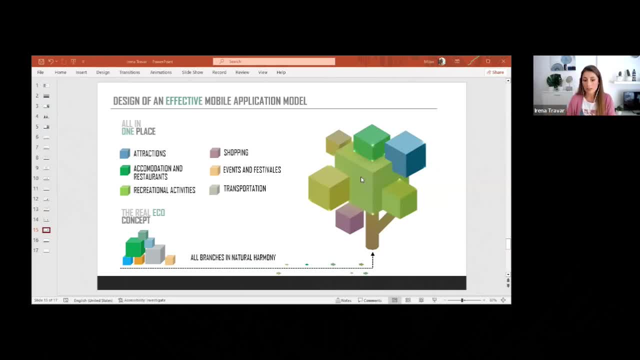 in architecture. okay, then i will tell them more about architectural styles in country influences and etc. so actually i try to um to really listen and feel their, their reactions, so of course i receive a positive review. of course it can happen that sometimes, whatever that you do, tourists are not satisfied. 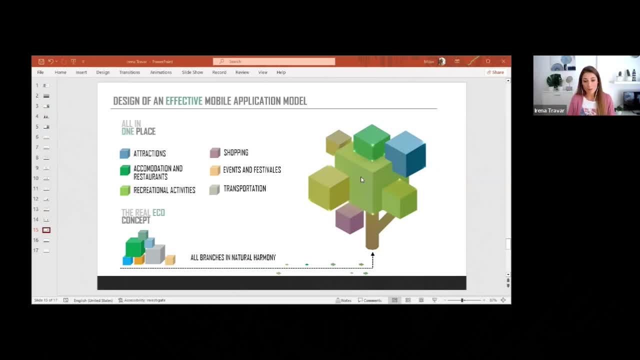 and you need to be aware that when you work with people, not everyone can be satisfied. it's not about only you. it's just that maybe you you haven't find a good energy between between you and and and the tourists if they leave a bad review, if it's only one review. 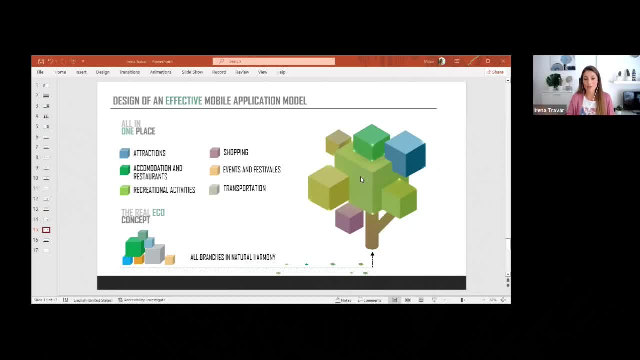 and you have 50 or 100 others good reviews, it's okay. it cannot influence so much. uh, of course, you really need to be um, to be aware that you did your best. that is what i was saying. okay, i really did my best and they, they wanted i don't know something special, like like nobody before. uh, 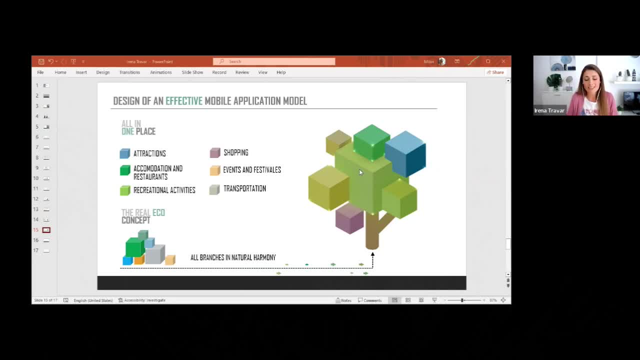 it's, it's really something that that happens, but it it doesn't, um, it's important that it doesn't happen and that's why i encourage you. so, uh, actually, uh, if you start working as a tour guide, you will have maybe three tours a day, sometimes four tours. okay, if somebody is is unsatisfied. 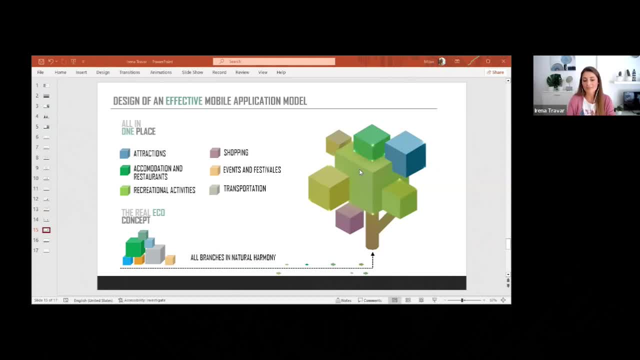 okay, if 90 percent are satisfied, then you do a good job. that's right. that's a great tip, irena, and the only thing i would ask emmanuel, is always reply to the review, first of all acknowledging whatever you know the complaint might have been. and uh, and you know present that, uh, you know the. 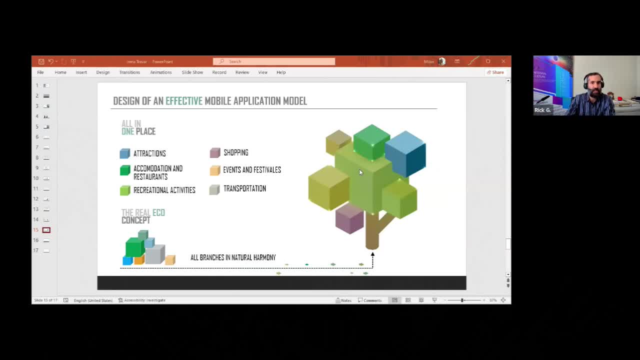 you'll what steps you might take, uh, to make a better experience next time? and, you know, maybe the person will consider revising. so thank you for that. and last one, because we're at the end of the session, let me ask on vishnu pandey, please, uh, let me ask you to unmute. thank you very much, doctor. 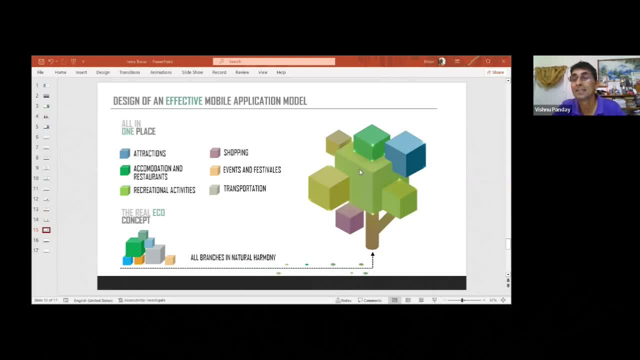 um, this is vishnu pandey, from guyana, south america. um, i'd like to offer a comment on the uh influence of tourism, so to speak, on religion. um, in guyana, you would know that? um, you ought to know that we have three main religions, that's, the christianity, muslim and hindu, and um we find that. 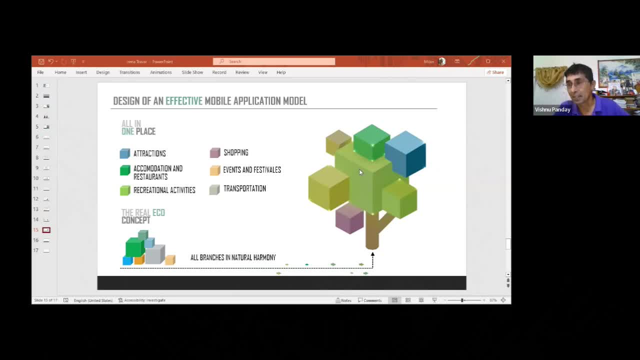 the influence of tourists might have a positive effect, as some, in some cases, are true in that regard, um when, for instance, in hinduism, we have several denominations or several beliefs, um or several characteristics within that hindu religion, and when people come from india for 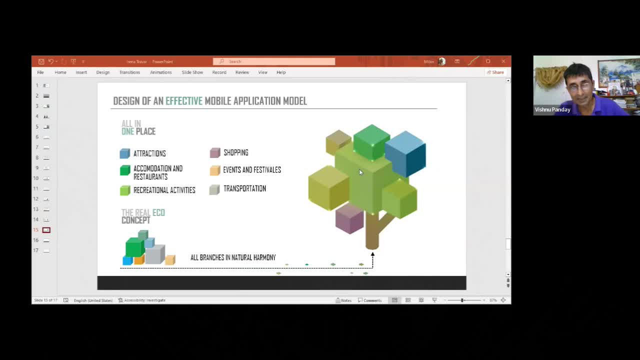 instance, they offer um ideas to the practicing of the convictions and that in the religion. so so, when they offer ideas, perhaps it's a best practice in the way we worship, for instance, and, um, that might be a positive influence on guineas, because, uh, you tend to to think that, hey, maybe i'm 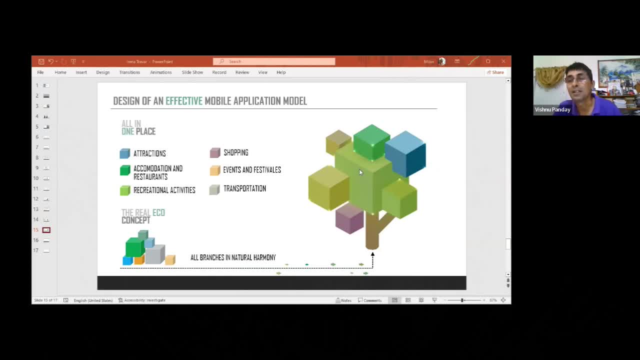 this is an interesting way to do what i believe in, and i and you want to go practice it, and so it is with other religion too. so i see it as a as a positive influence. while not interfering with the conviction- um potent conviction in some cases- it also can lend a perspective in the way we practice. 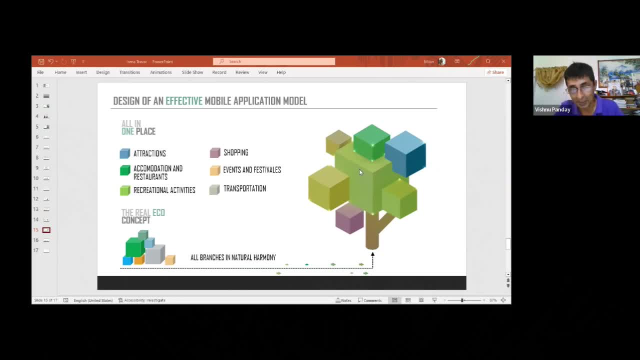 or perhaps the way we interpret some of the doctrines in the religion as well too, as you know, as opposed to Lecter, and so, um, we think that the, the connection between, uh, the both of those, uh, you know, and, and this, for me, is that the link to the, the significant things that I know, the 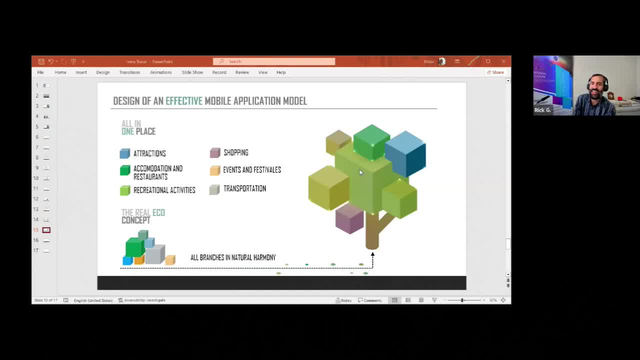 очкуes and the interpretations that i saw in the texts and, uh, you know um we, we, we see evidence in Guiana. i'd just like to share that, thank you. thank you very much. okay, fantastic, uh, did you want to comment on that, irena? uh, well, uh, uh, i i, i didn't know that. 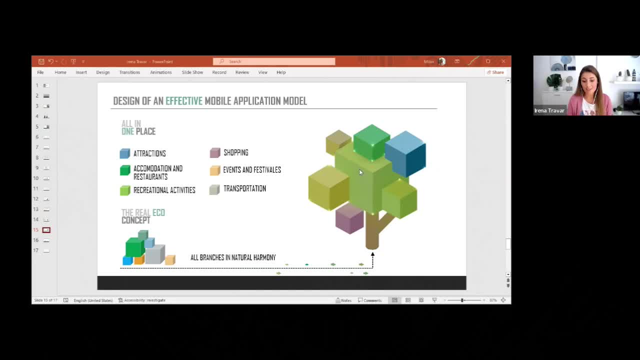 wanted to add that it's important that we share our experiences and nowadays, you see that, uh, for me, it's really amazing that, uh, that we can talk from many different parts of the of the world and always hear something new, something interesting, something that that, of course, can can give us some 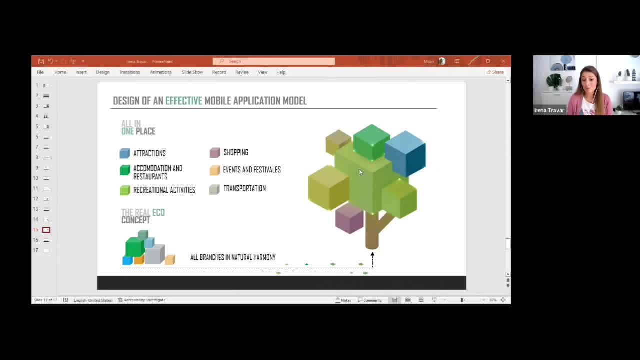 ideas for for our future virtual work, so to to be the the best versions of ourselves. fantastic well, thank you, vishnu, for that contribution and, irena, it's been an amazing- uh, you know, an amazing- live session with you and learning about the geotourism tourism and how i mean it actually turned into a. 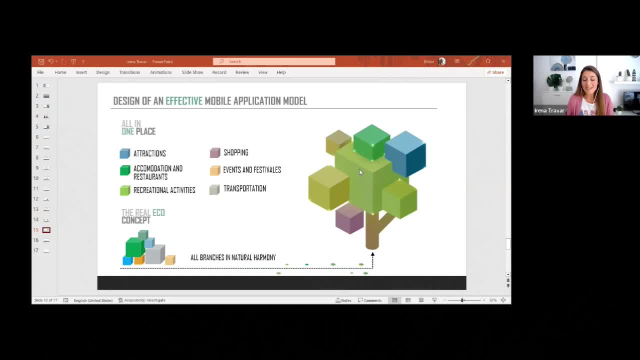 cultural, and you know religious and thing, which is also tourism. you know, you, you, you, you never, you never know, but uh, actually, uh, yeah, i i also wanted to to thank you, um ricardo, very much for for this invitation. uh, actually, i didn't do it at at the beginning because i had problems with my 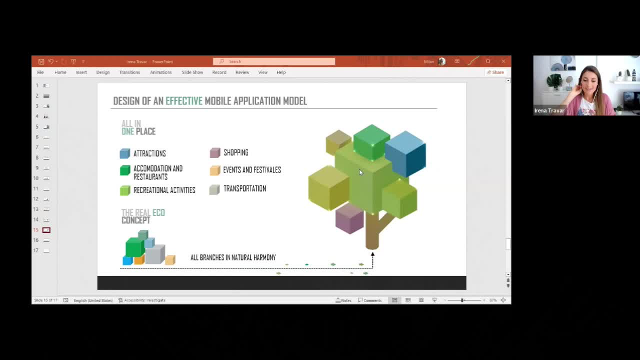 with my mic microphone. uh, so, uh, it's. it's really amazing that, um, i also made the concept of of today's uh presentation like something that can be interesting, uh, for for students in general, never mind from um, from which country they're coming, continent, or what they uh, what they. 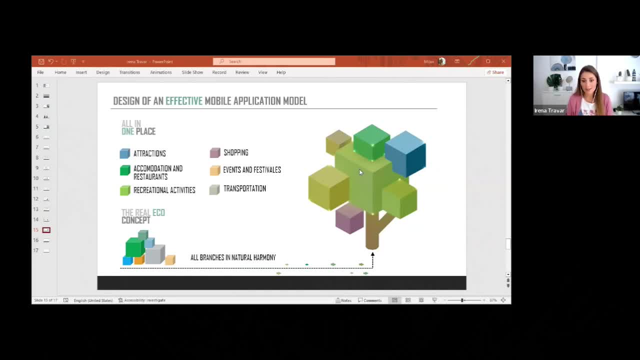 actually uh study, but something that that can help you in in your future life, in your in your future life, your future career- fantastic. well, we, we hope, uh, you can make time for us again in the future and uh and maybe do a second session and and subsequent sessions to help our students. 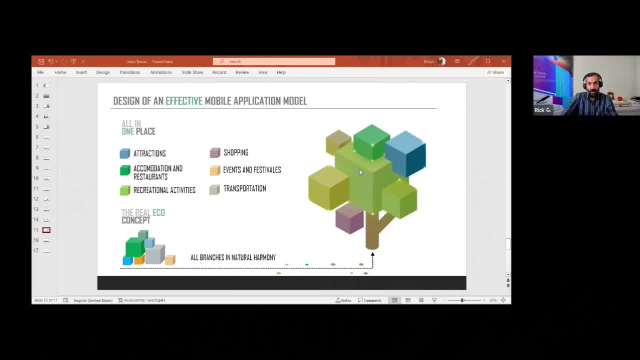 uh, you know, see how they can uh learn about eco, tourism, tourism and the different research that you're doing you. it's a, it's a great addition. we have 90 participants, so i think it's been a success and i really appreciate you making the time for us. thank you, thank you, thank you.